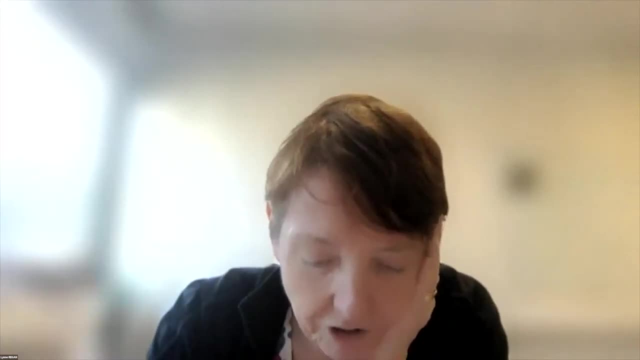 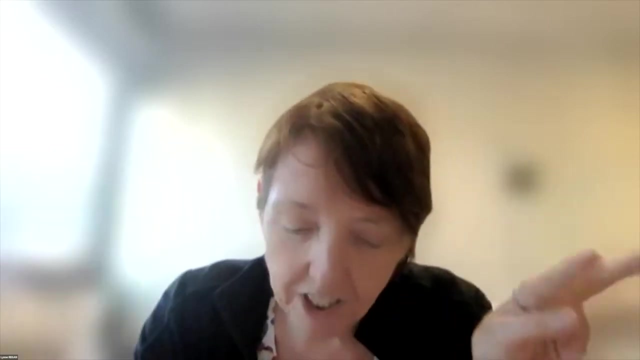 call it engineering rather than tinkering. I think we're a lot further along. So the goal is to do predictable engineering of proteins, And there have been some terrific successes, but there's a certain degree of subjectivity in protein specificness to those successes, And so in protein engineering, researchers learned from. 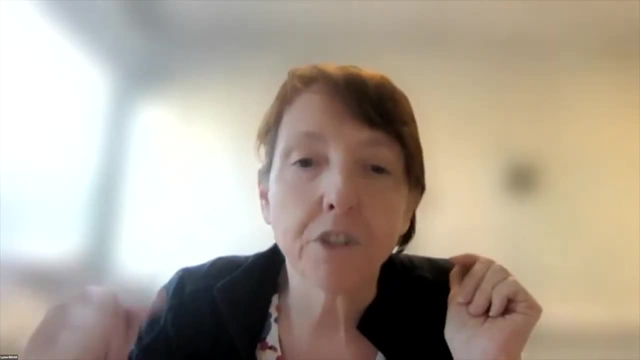 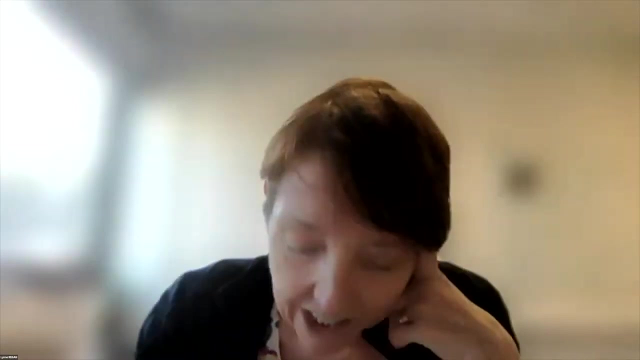 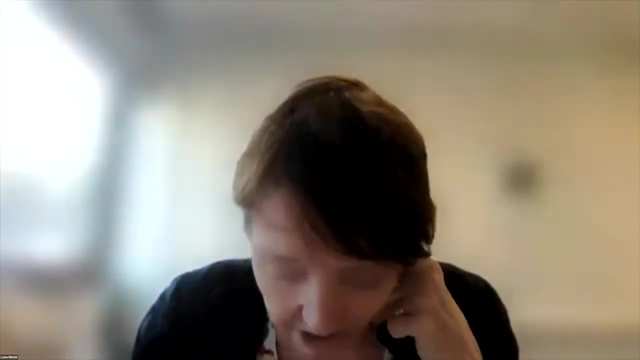 published data, But also, as you'll see from these three examples, go. they go into lab to actually make something new and to test it themselves. And in addition to testing fundamental concepts, then we're also making progress towards practical products. And I think, Giovanni, at the end we'll 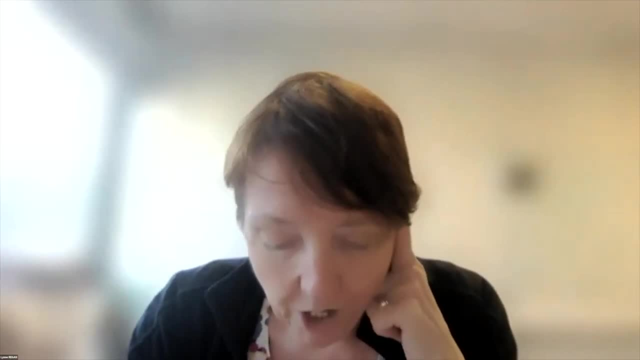 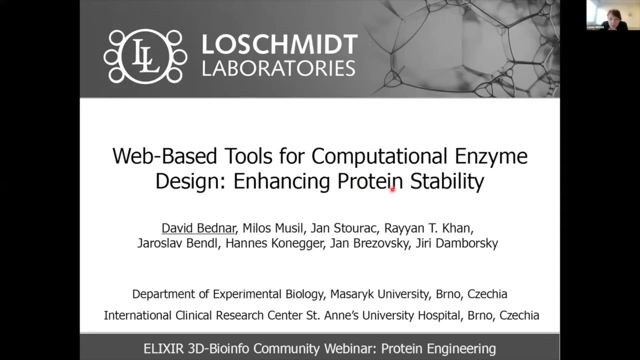 be talking about one particular example of that. But, to start with, our first speaker is David Bednar, And he's going to talk about what are some web paced tools that are available to you and to tell us about how his group has used them to do things in the area of protein design. 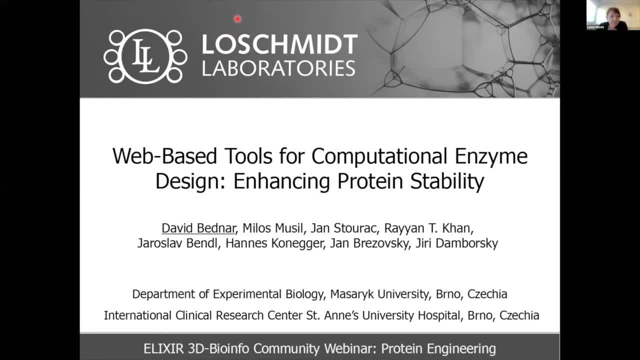 So over to David, thank you. Okay, thank you very much for kind introduction. So good afternoon ladies and gentlemen. my name is David Bednar and I'm from Walsh-Mitt Laboratories at Masaryk University in the Czech Republic, And in Walsh-Mitt Laboratories we focus on protein engineering from different points of view, both like 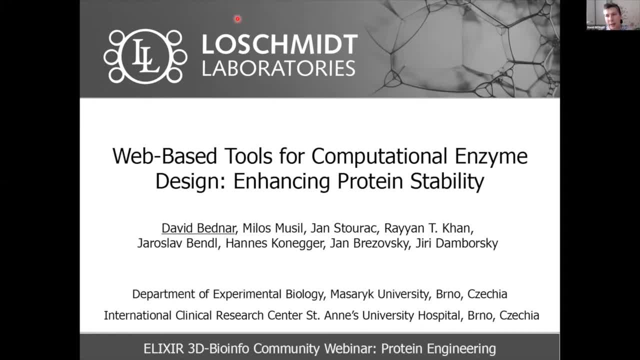 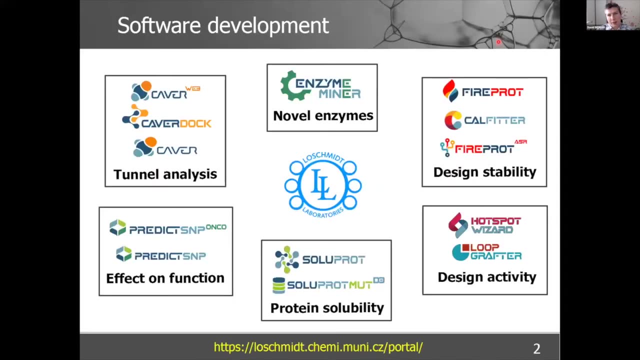 experimental and also theoretical, And in my team we focus on molecule modeling and bioinformatics and also on development of computational tools, which I want to talk about here also. In past few years we have developed quite many tools- It's actually 12 tools and two databases- but there's not enough time, of course, to talk about all of them here, So I'll focus mostly on two of them, which we'll consider mostly design of protein stability. 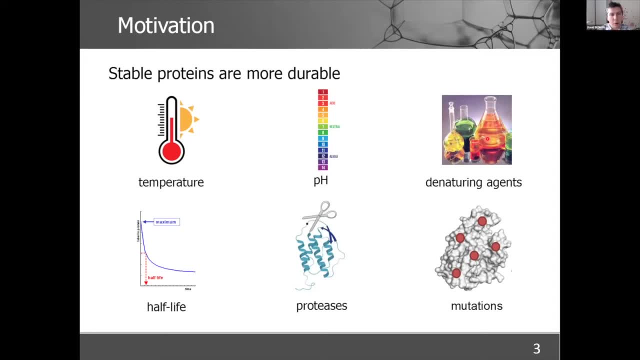 I don't think that I need to really go through the motivation much more thoroughly, because we all know that stability is one of the basic properties of all proteins And if you want to use your protein, And if you want to use your protein, 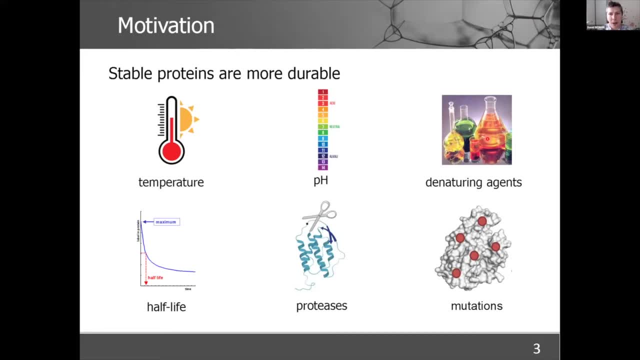 In both basic science or or in some applied technologies. you need to have proteins stable enough And if you have stable proteins, they can withstand much like withstand very, very difficult conditions like high temperatures, pH, and also additives like denaturating agents and so on. 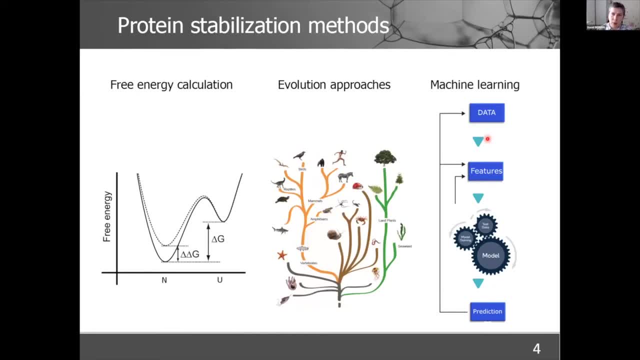 think we can divide it into three categories. first is calculating all the fall of the folding free energy, so based on some force fields. second are approaches that are based on evolution. 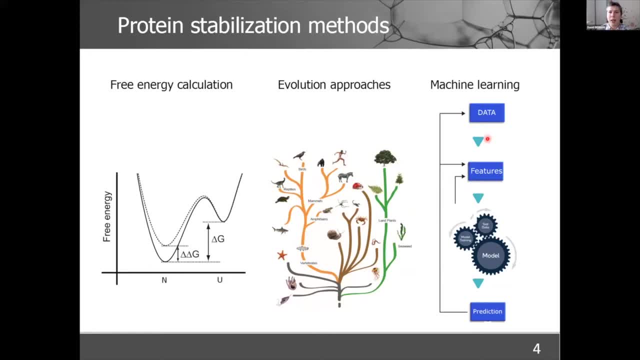 like consensus designs or ancestral sequences. and last one is based on machine learning, where you're trying to find some, uh, some statistical, uh interesting stuff in your data. i want to focus here mostly on the two first two categories, so the free energy calculation and the evolution approaches, because for both of them we have developed web servers that can. 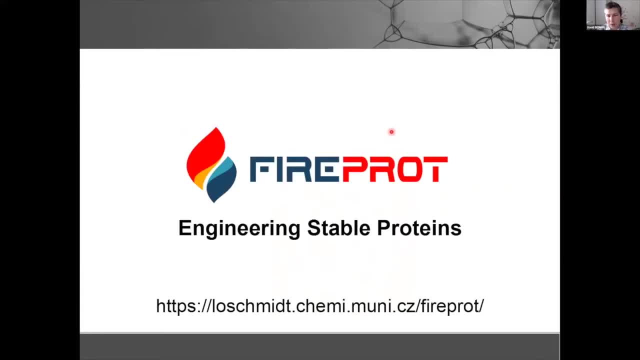 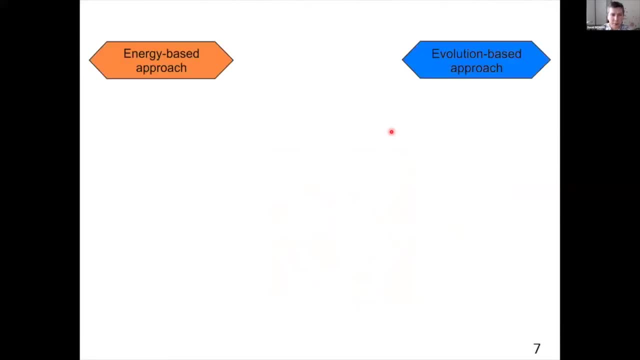 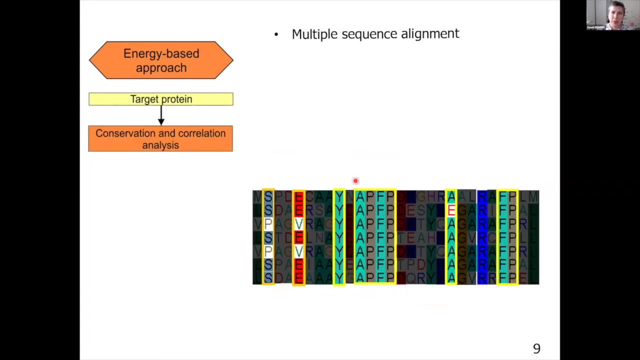 be used. so first of all i will start with fire prod, which is the web server for engineering stable multiple point newtons. it's divided into two different strategies and the first one is based on the energy output approach, where you take your protein- a protein of interest- and you construct multiple sequence. 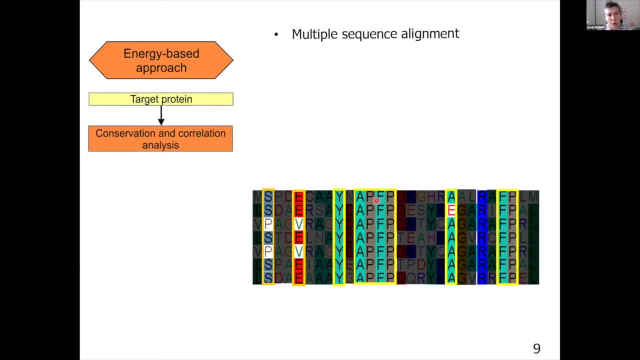 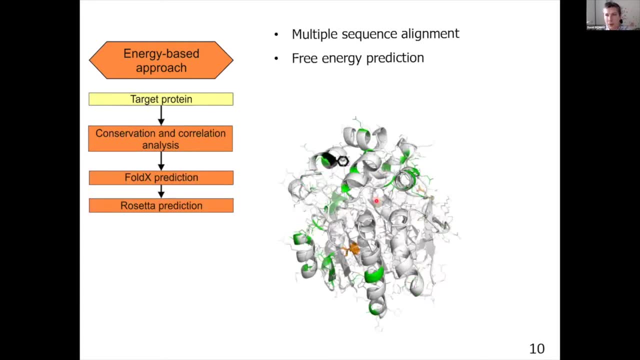 alignment from homologous sequences. you discard all the conserved and correlation correlated positions and then you go for the for the analysis by two different tools which predict the free energy of unfolding, and these are foldex and rosetta. so we calculate all the possible single. 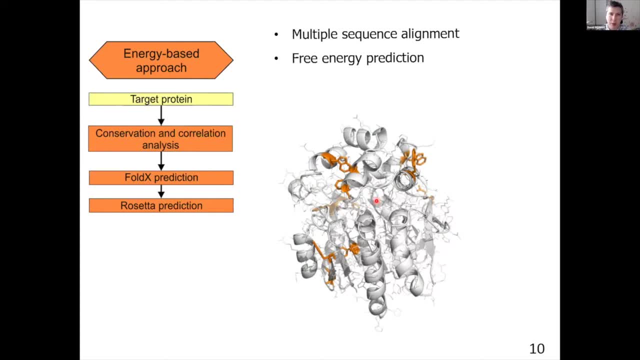 point mutants by these tools and everything that passed some energetic criteria, some some cutoffs is, is going to the next next steps. we also check some of the important interactions, mostly like soul bridges, which we know that are not predicted well by these tools, and we also construct all the possible double point mutants. 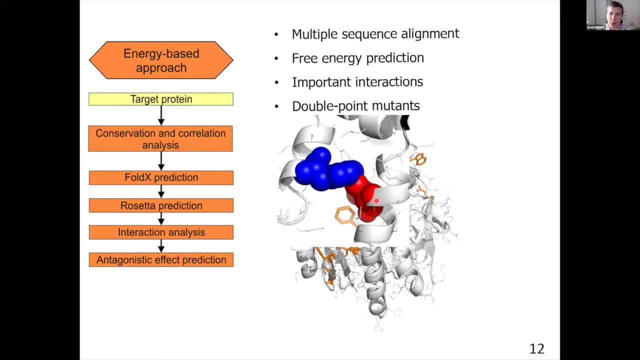 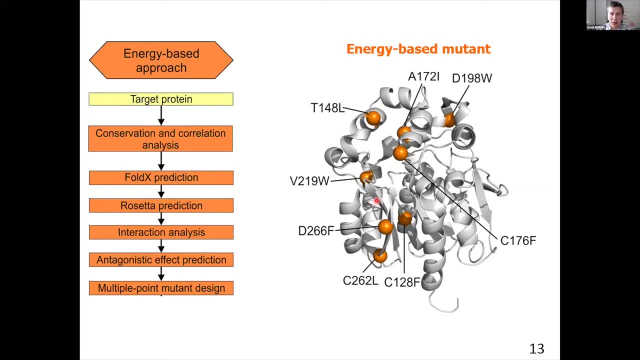 to see if there could be some antagonistic effect to filter also some of these mutations. so all the mutations in the end that pass all these criteria combined into the multiple point mutant which has really a good chance to gather only the stabilizing mutations and discarding everything that could be that could be. 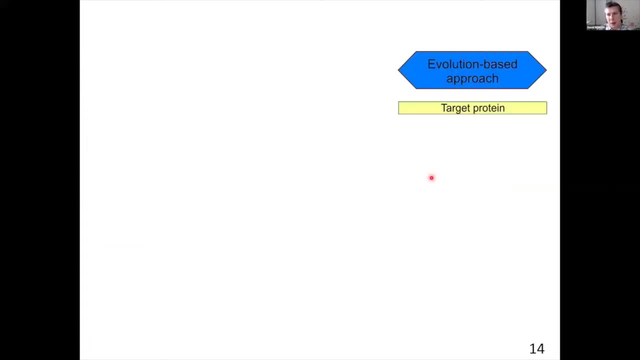 tricky. we also saw that these energy based approaches or force force field based approaches sometimes fail to predict some kind of the mutation. so it's very uh useful to add also some evolution-based techniques to complement the mutations that you're going to see in the next steps. 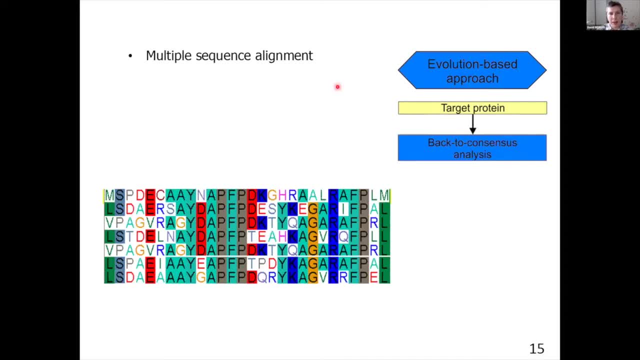 so we're going to start with the same protein again. and then the difference. the main difference is that we don't calculate the free energy here, but we select the mutations or create a pool of mutations by the back to consensus analysis. so we construct the multiple sequence, alignment and 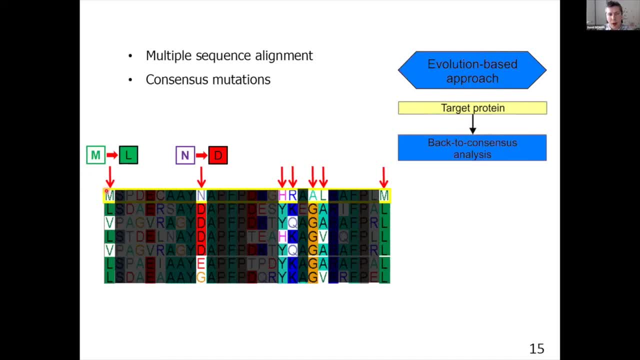 we are trying to find those positions that are not conserved in your sequence, but we are trying to mutate them into the most conserved residue in that particular sequence. so we are going to start with the first one, that is the particular position. so by that we get we have quite nice pool of 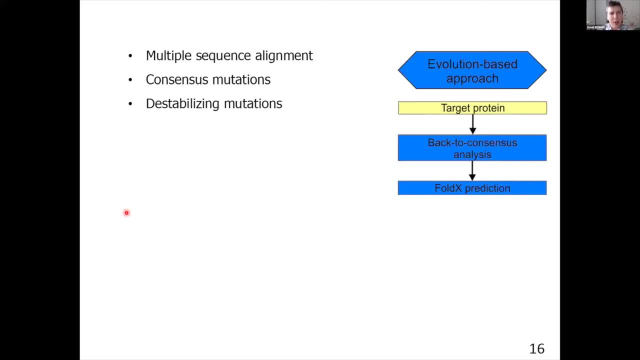 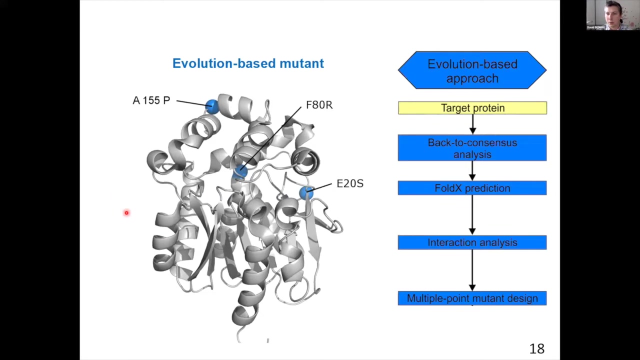 mutations and then we go some through some filtering- filtering steps, as in the previous case. so we calculate some destabilizing mutations by full decks. we also check the interactions that are important and in the end we provide the user with another multiple point, newton, which is based 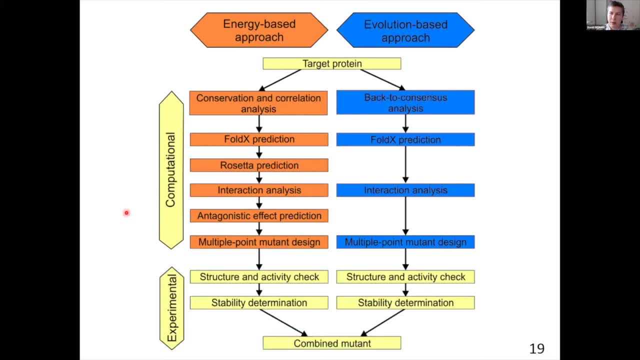 So altogether this is the computational part. Then usually we synthesize the genes and we check them in lab. So we check the structure stability activity. If both of the mutants are okay, then we combine them here into the combined multiple point mutant. 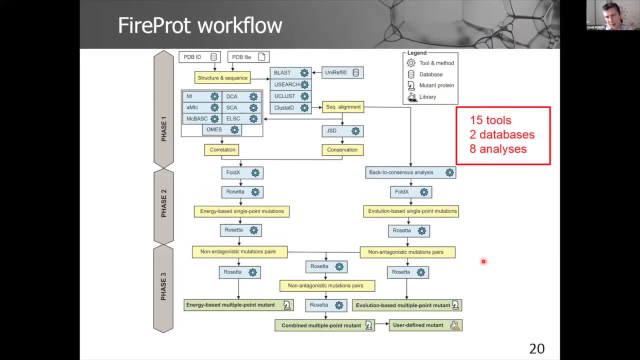 But the workflow seemed quite, quite difficult. You can see that it consists of 15 different tools and two databases, So just installing and going through all the analysis is quite demanding And for people who are not experienced in bioinformatics this could be really overwhelming sometimes. 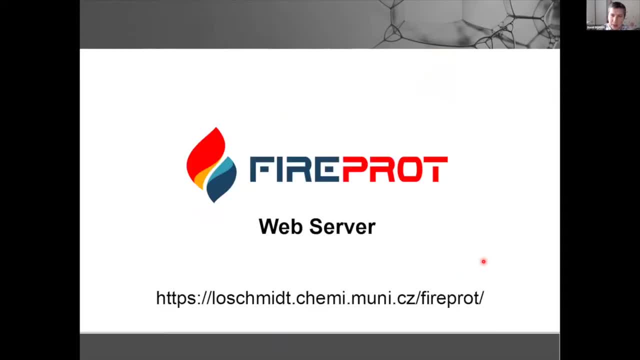 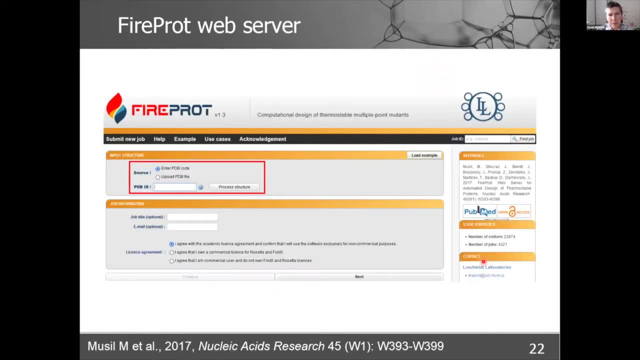 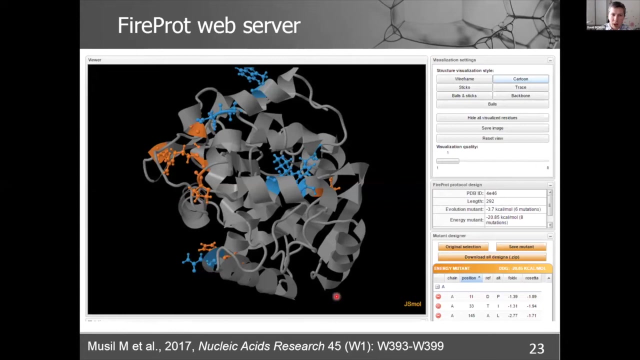 Therefore we decided to go also for the web server, which could be easy to use with nice graphical users. So in the end the only mandatory input for the FireProt is the structure of your protein. So you upload it here And then, after usually a few days of calculations, you get the output page where you can see the mutations mapped on your protein in this visualization window. 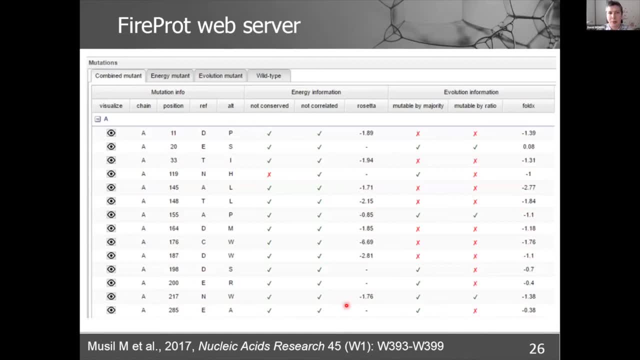 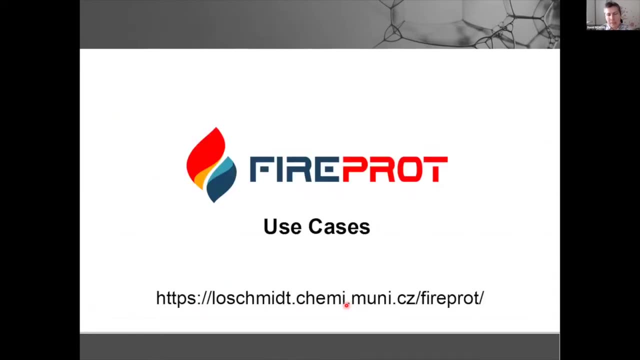 And below you can see a table with all the suggested mutations that should have the stabilizing effect. To show you also that the method really works, I selected a few of the proteins that we stabilized. Actually, we stabilized already more than 10 different proteins. 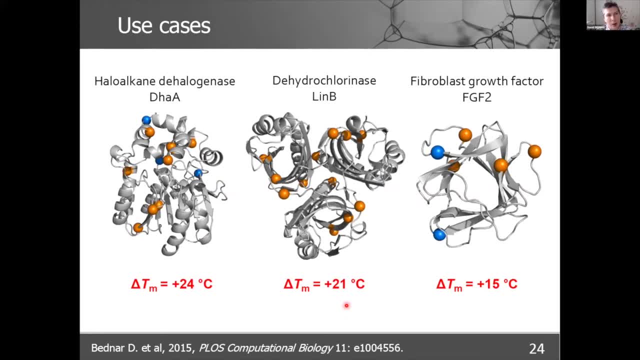 But here are some of the selected: halal: candelogenase, DHAA, the hydrochlorinase and fibroblast growth factor 2.. You can see that for all of the proteins, we were able to select a few of them. 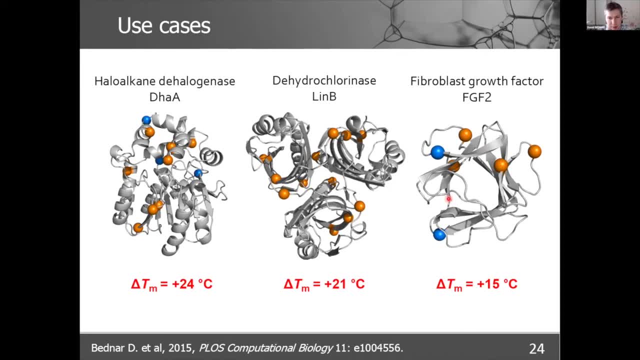 So to stabilize them for more than 15 degrees of Celsius, still keeping their biological functions. In the first two these are enzymes, so enzymatic function was conserved still, And in the third case it was actually a very interesting case where this is the protein important for proliferation of cells. 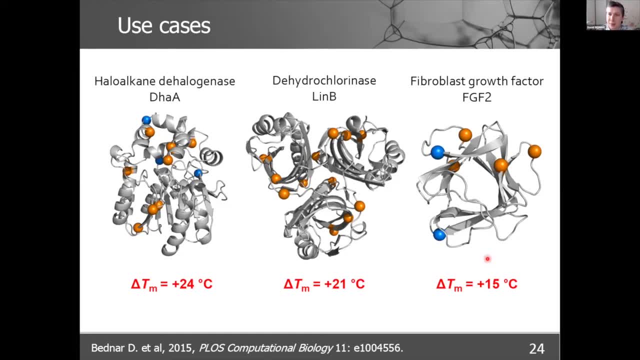 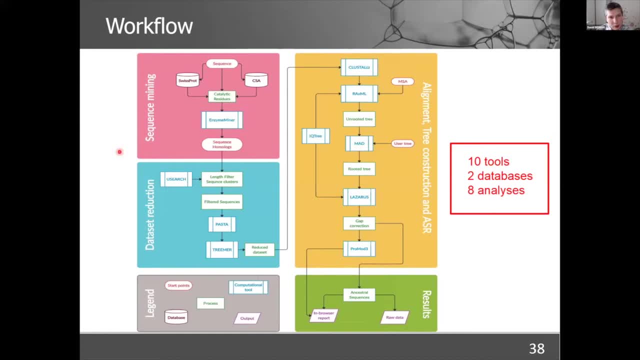 So this protein can be really used because it has a lot of protein in it. So this protein can be really used because it has a lot of protein in it. analysis and all the all the parts like sequence mining, filtering and data set reduction, multiple sequence alignment, construction and the evolutionary tree- all these things were in. 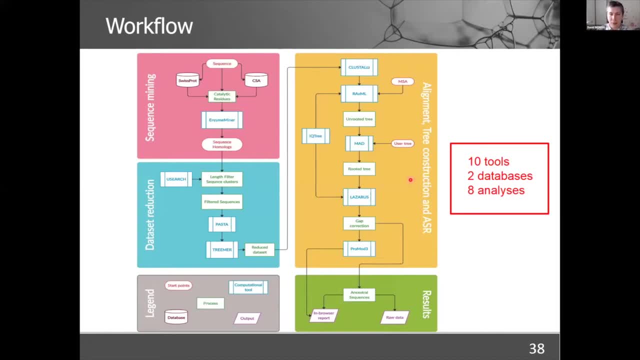 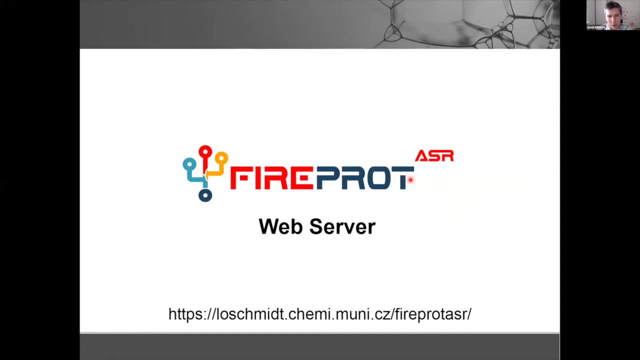 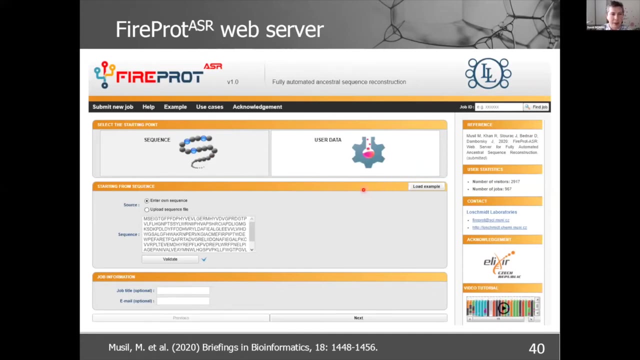 the end automized, so so it can be easily used. so in the end this web server was was developed and it it looks quite similar to the classical fire prod, with the only difference is where you can see here the sequence instead of the structure as the input. so just the faster format is enough. 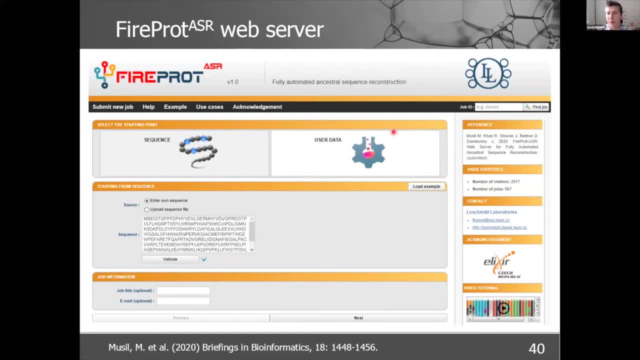 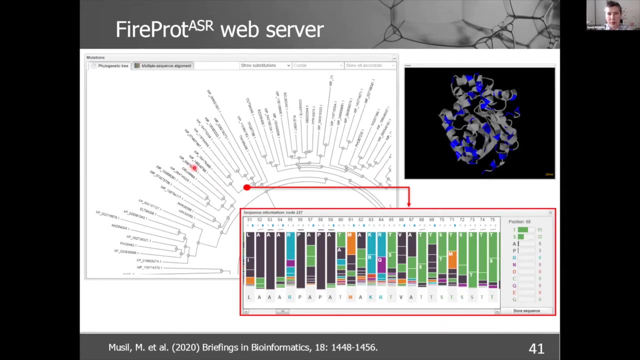 to start the calculation. of course, user can provide us with some other other information that he has available after submitting this job. usually after a few hours you can get this kind of tree, so the three of the homologous sequences of your protein family and you can select any. 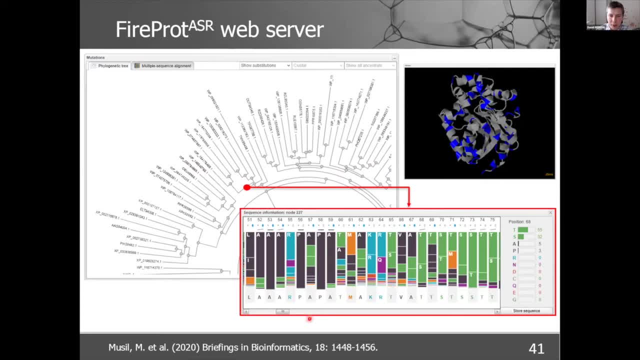 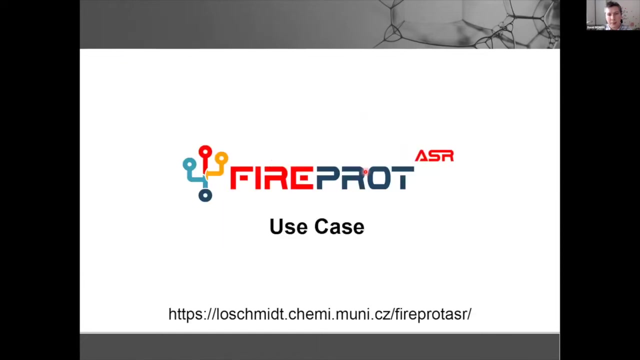 node in that tree and you can. you can visualize the, the sequence with all the posterior probabilities, like you can see here. and also we build the homology model to visualize all the differences between your wild type protein and this particular ancestral here in the visualization window. so you can see that, starting with this one, there's an opposite component of th and this one. 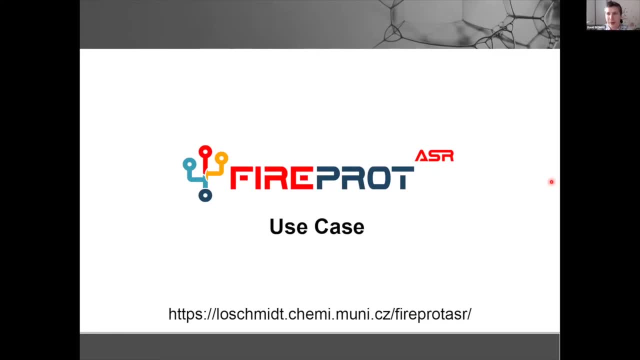 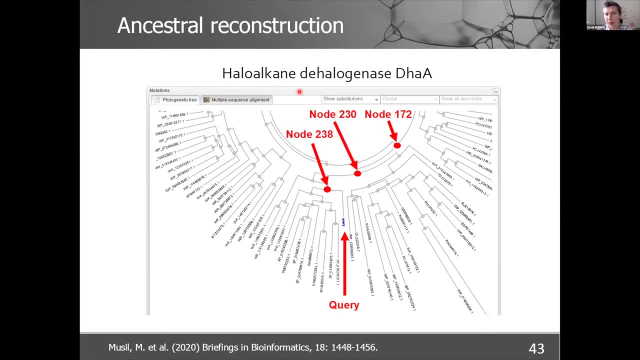 here, for example, we don't have any枝, but it's just the same formula, so you can see that it's a little bit different. but yeah, we have to start to. don't be afraid to start to work with it. we have to learn some of the three components anyway. so we're using a leveled method and we 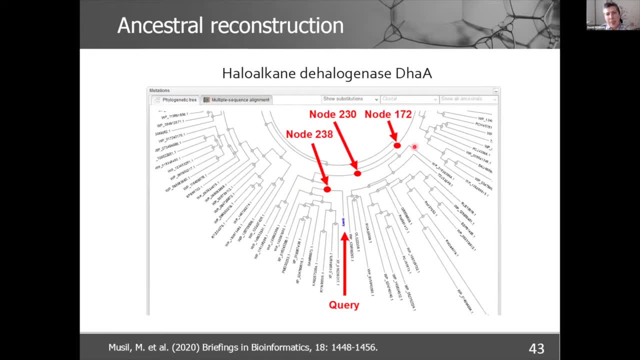 we have to learn the protein layout and this method is actually actually useful and it can be can be used. it's quite robust. uh. we applied applied it on on the uh helicon, the halogenase family. more concretely, it was the dha enzyme from rodococus. 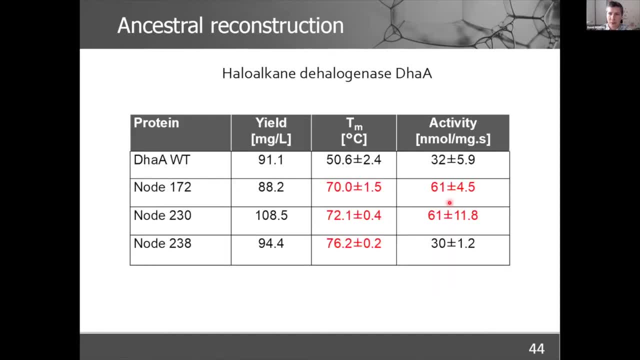 So we synthesized genes, we went for the cloning and testing of the proteins in the end, And you can see that all the proteins had quite nice yields, which is also very, very common for ancestral proteins. You can see that all of them were nicely stable. 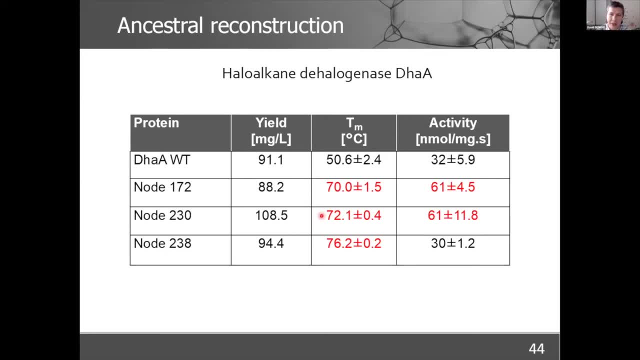 The melting temperature was increased for at least 20 degrees of Celsius, And some of them have even increased activity to the double that was in the wild type protein. So, as you can sometimes hear some people say that in the past everything was better. 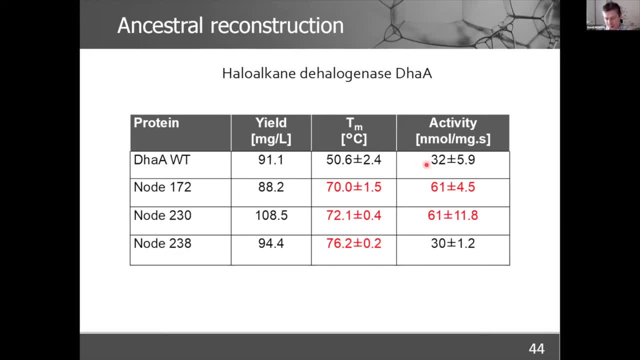 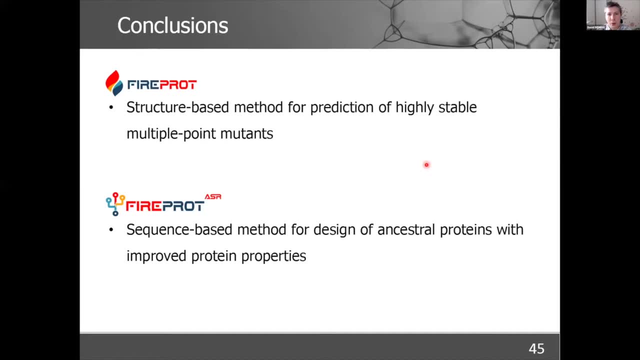 In the protein world. it seems like it's kind of true. So just to conclude my talk, I wanted to show you these two techniques, Two tools for protein stabilization. One is FireProt, which is a structure-based method, where you need the structure to get the highly stable multiple-point mutants. 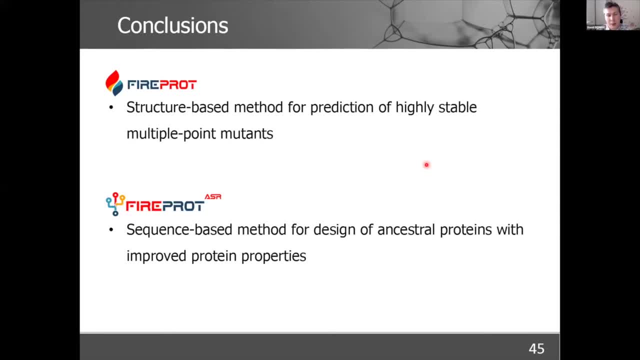 If you don't have any structure, or even if you have, you can still try to use the FireProt ASR, which is useful for phylogenetic analysis and also for stabilization of your protein. just based on the sequence, All the tools. 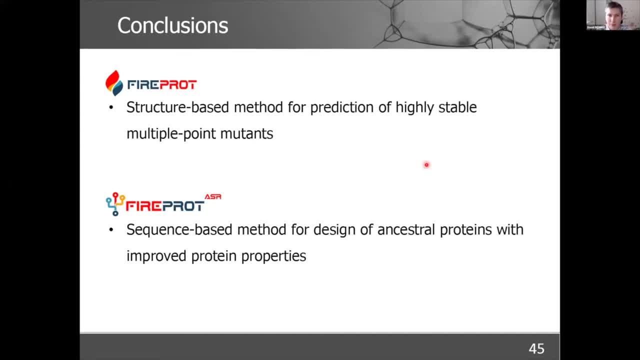 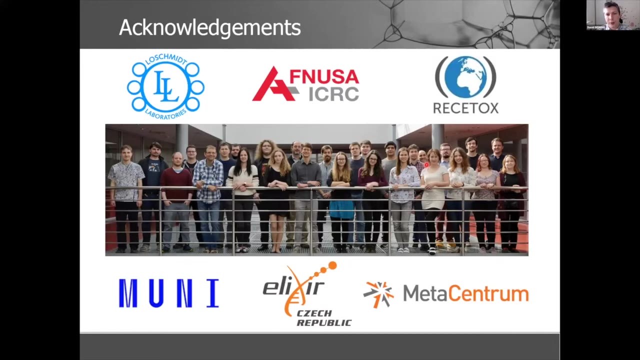 We try to make really easy to use for experimental biologists, without the necessity of having deep knowledge in bioinformatics and without installing these tools. So this is all from myself. I would like to thank all these institutions for financial and computational support, and also to our group of Lushmit Laboratories. 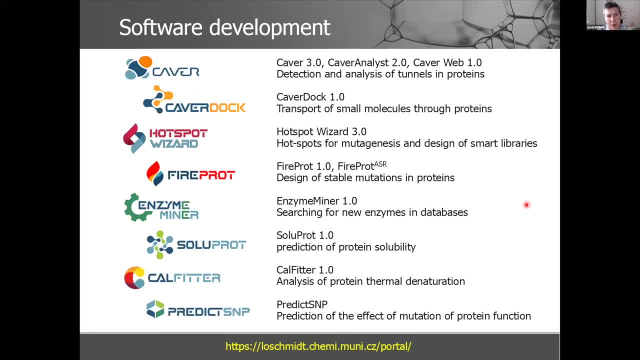 And I'll end my talk here- on this slide where you can also see some other tools. So if you are interested in tools for analysis of protein and protein design, you can go to this page down here. Lushmit Chemik, Muni CZ, slash portal. 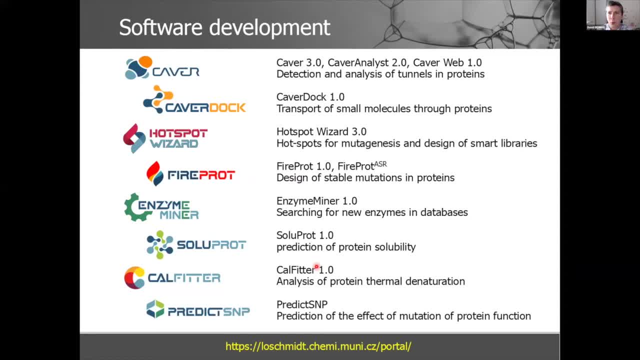 So thank you very much. I'll be glad to answer some questions. Thank you, That was terrific. We have. you can put questions in the chat or the questions and answers. I just saw another one I have. I'm going to read the odd one from the chat. we're going to have more chance to discuss this at the end. 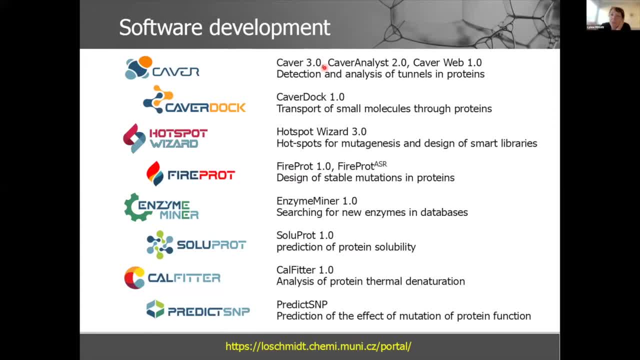 So this is an easy one from the chat with what. what's your experience with metalloproteins or proteins that have got metals in them? Does everything you've said work equally well for them, or are there any caveats with that? Yeah, if you, if you, have some metal protein, this could be quite problematic for the file product itself, like the structure based tool, because you need to, you need to parallelize it. 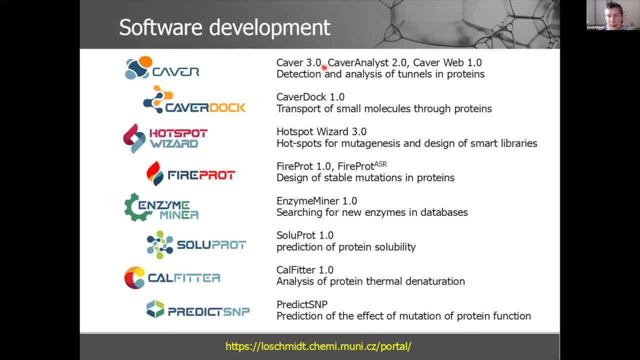 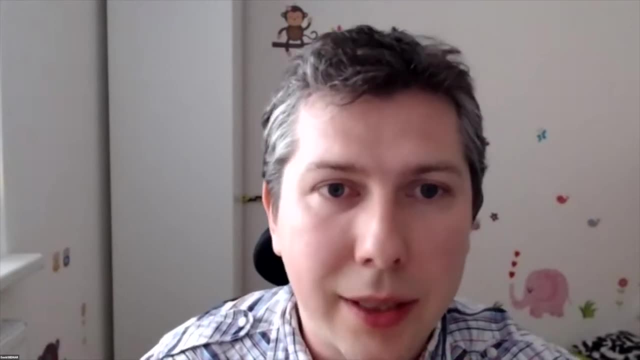 So you need to, you need to parameterize, parameterize the cofactor, And this is usually not not very easy and straightforward for for for this automatic method. so so it's not possible to run it in the fireboard itself, but the fiber of ASR doesn't care much about, about the cofactors. 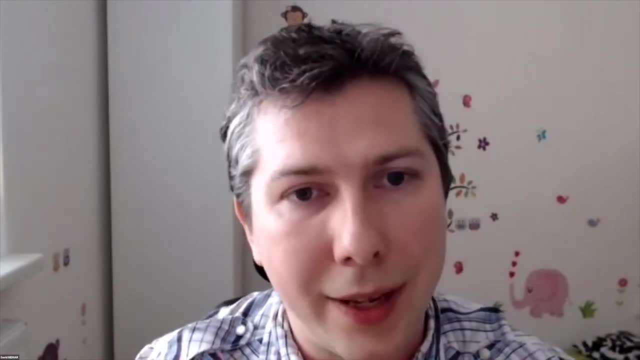 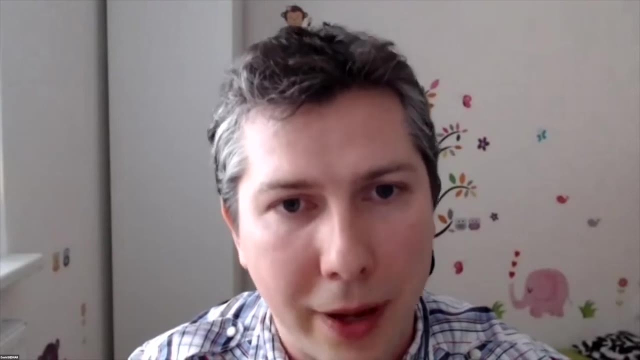 Yeah, those, those amino acids that are like keeping the cofactor in place are are usually conserved, so they are not mutated at all. And and and, uh, this fiber asr can be used even on metal proteins very easily. okay, i have one question. 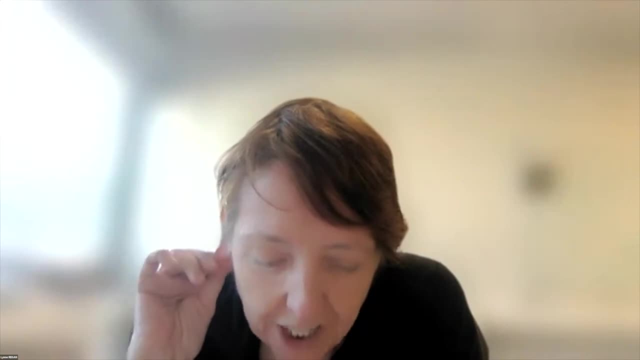 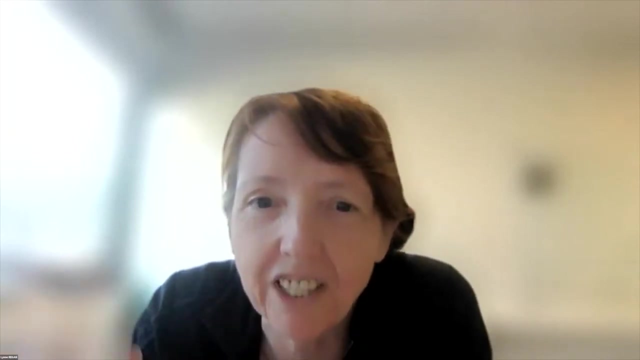 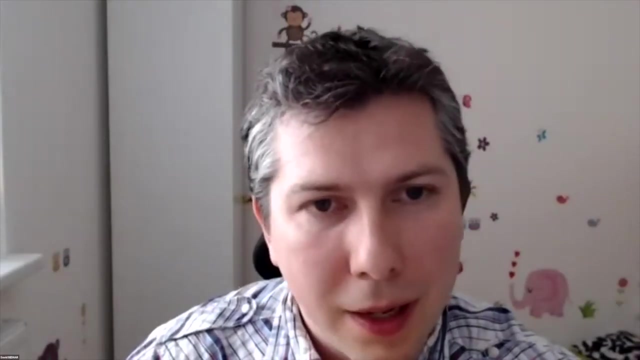 which was what's going on with that node 238, protein, new shoulders- which has a tm of 76 but then an activity of 30.. do you have any? you must have looked into that because it's quite different from your other examples. uh, with this ancestral sequences, you usually uh have really a lot of. 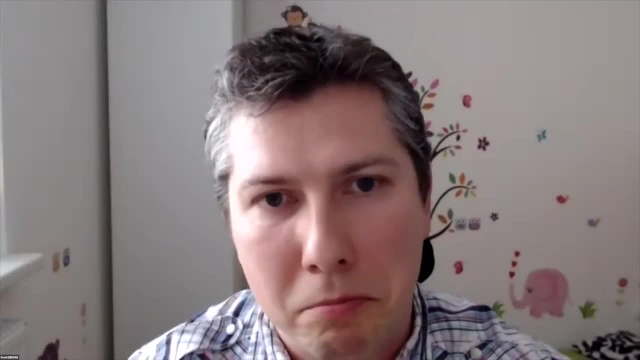 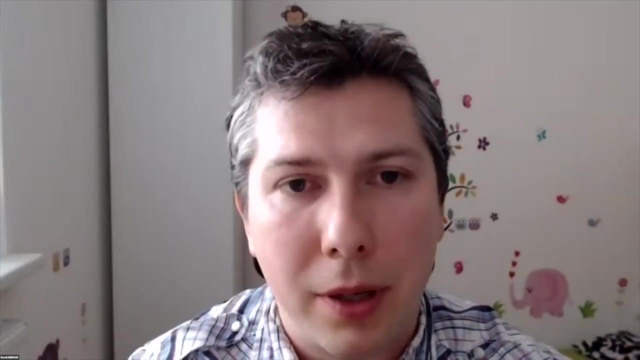 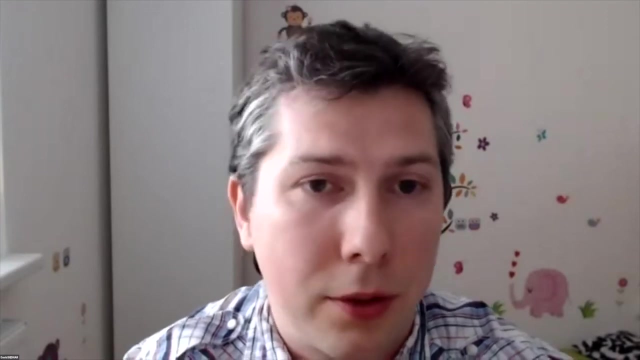 mutations in your protein. yeah, it was usually tens of mutations that we that we constructed there. still, on the positions that are usually variable, uh, the activity of of that particular node you mentioned is actually the same as on the wild type protein. so so there was no, no problem with the. 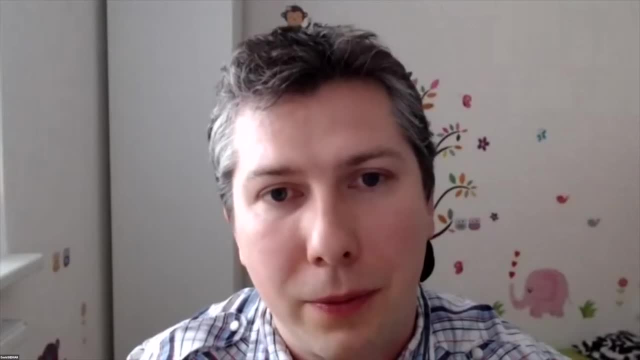 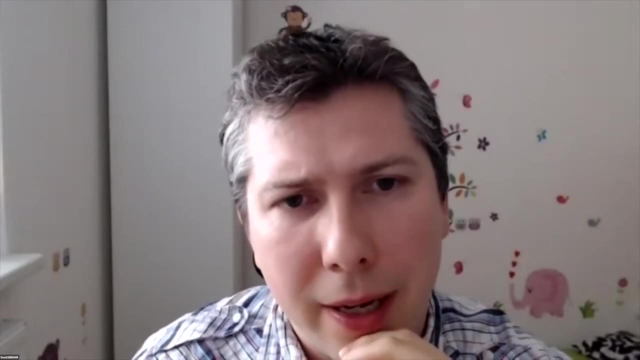 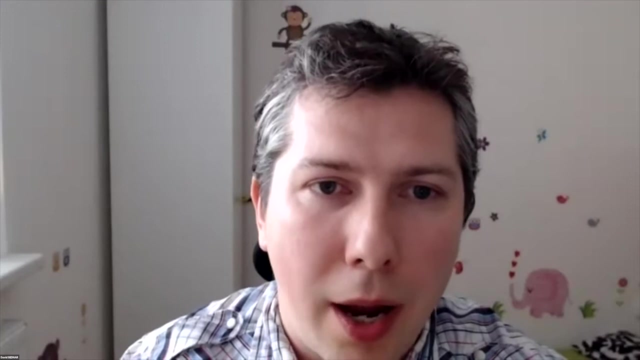 protein. it's just not as good as for the. for the others, i actually had also some some extra slides, uh, where, where we tested the substrate specificity of these ancestral proteins and those were quite uh quite interesting because they have much broader specificity and usually we even see higher. 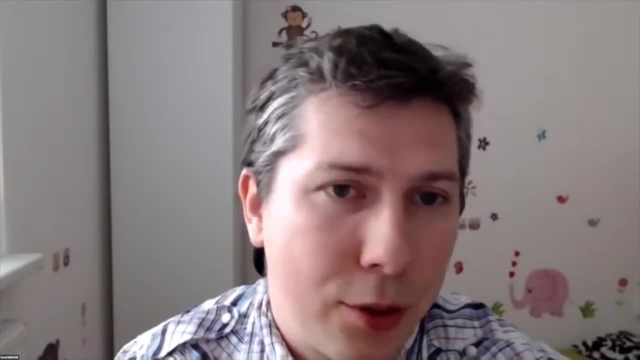 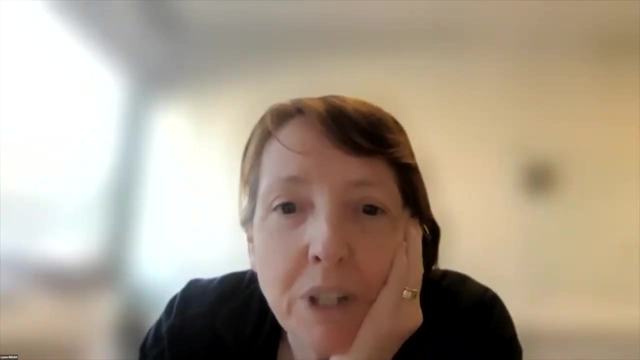 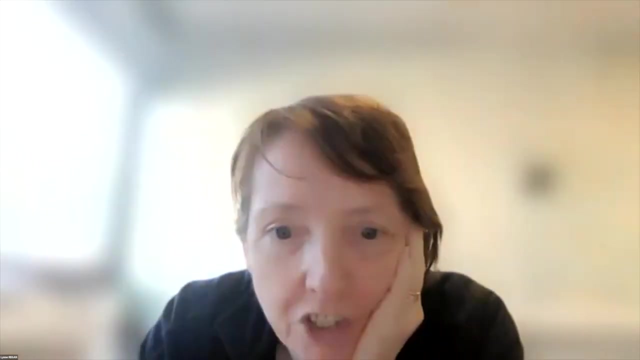 activities for some of the substrates. yeah, so, so there's no, no, no problem with that particular node. it's nicely stable and activity is fire. so i am just we. i'm gonna not read out any more questions. we're gonna save them for our discussion at the end, even though we have a bunch. so keep putting them in, people. 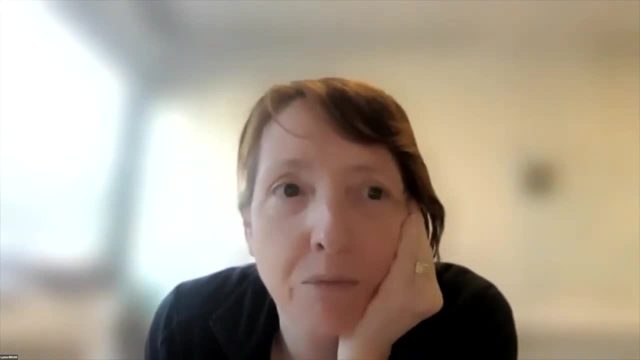 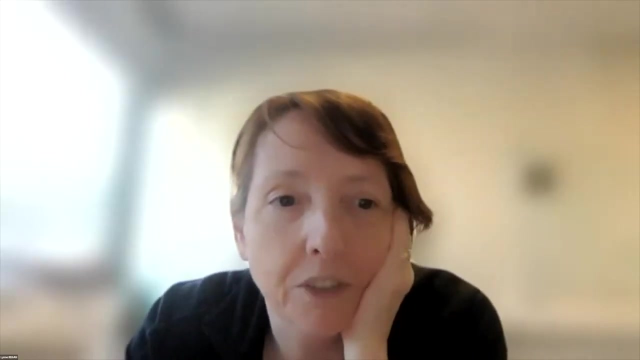 i would like to move on. thank you for a terrific presentation and for sharing those tools with the community. i'm going to move on now to chris wood, who's going to talk about um, how to rank designs and compare that with experiments. so i'm going to 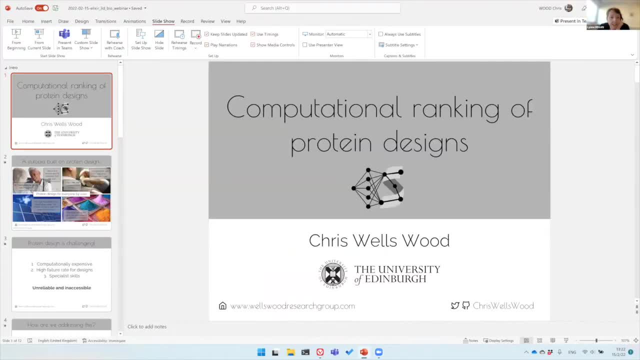 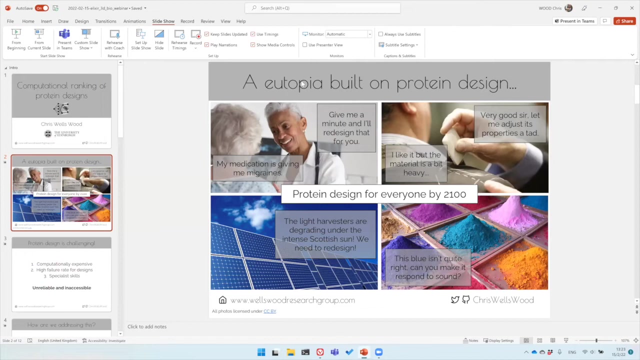 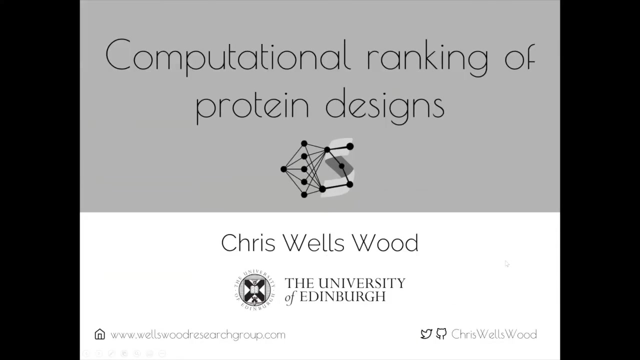 to Chris And, as I said, keep putting things in the chat. Oh, hopefully you can all hear me. Yeah, it's good. It's little thing is over here. Okay, Hi everyone. I'm Chris Wood. I'm a lecturer at the 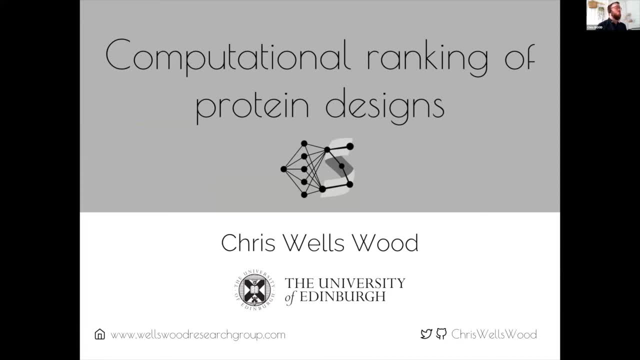 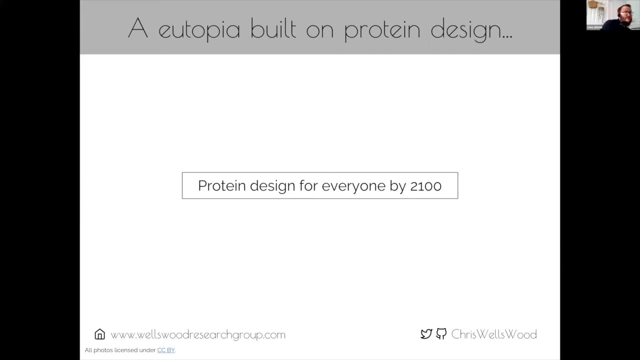 University of Edinburgh and my group's interested in protein design and protein engineering And one of the aspects of our labs is evaluating protein design. So I'm going to talk about that a little bit today. So I'm going to start off with the big picture stuff. This is the group manifesto. It's what. 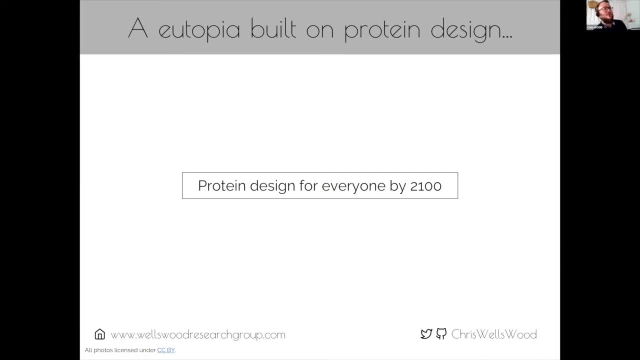 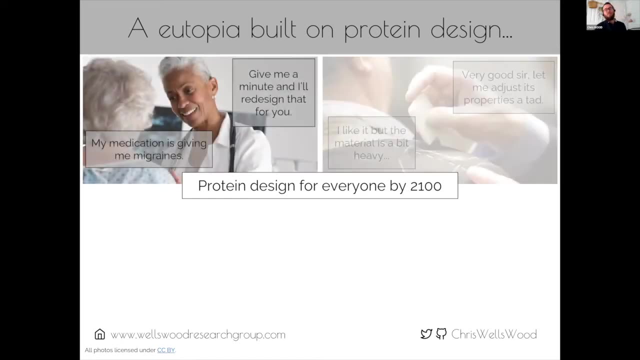 we're sort of aiming for, And this is a utopia built on protein design, And what we'd like to do is to enable everyone to design proteins by the year 2100.. And this is, I really mean everything. So maybe it's your doctor who's providing some protein based. 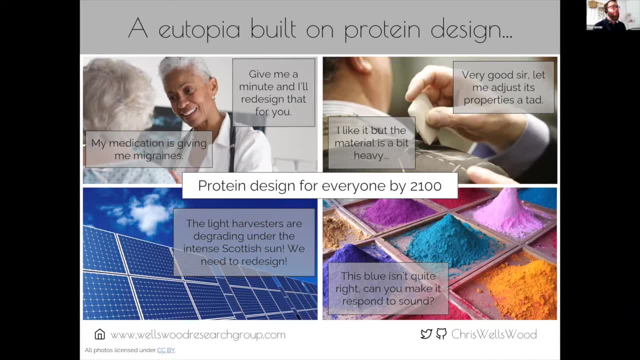 therapeutic that you've got some unintended side effect from and you redesign the protein in order to minimise that side effect. Or maybe it's a tailor who can tweak the properties of a protein based materials, like rules, in order to make it more suited to clients needs. or it's maybe light harvesting proteins. 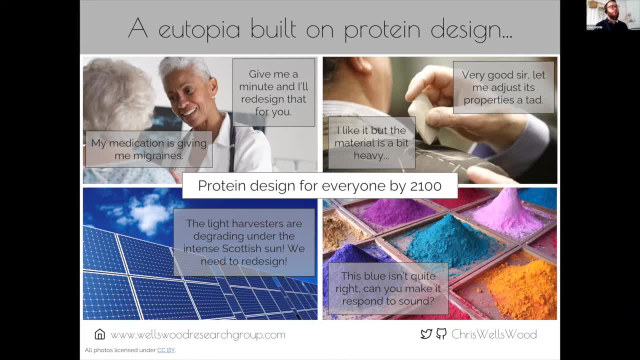 in some solar cells that needs to be tuned to the environment that they're being applied in. or maybe you know pigments that an artist is using that they're a protein based pigment and they want to change some of its properties to make it more useful. Now these examples. 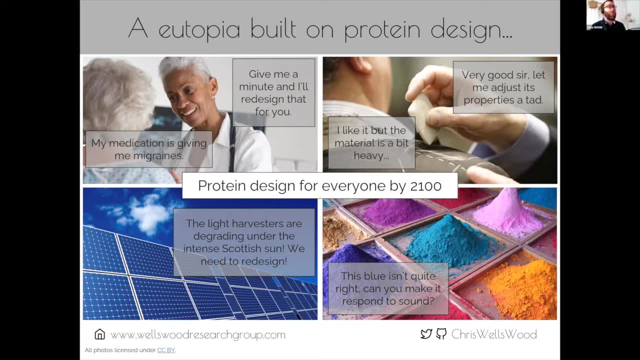 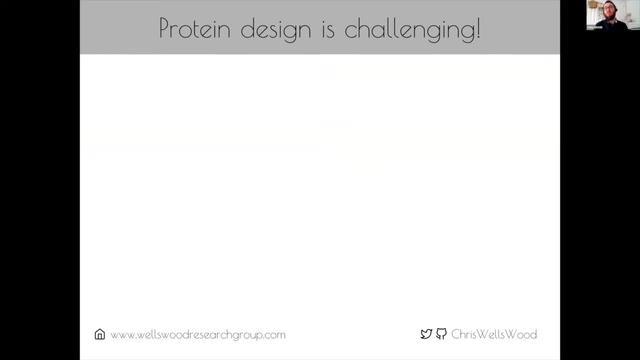 they're tongue in cheek, but these are all areas where proteins are incredibly important. At the moment, there's companies that are developing around all of these sorts of applications, But the truth of the situation is that protein design is highly challenging. So it's it's computationally. 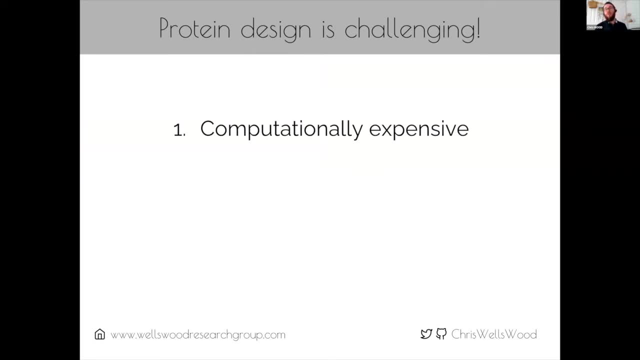 expensive And certainly you know, the more compute that you throw at the problem, I think, the higher that your success rate is and this is fair to say, it's also there's a there's a very high failure rate. So even in the very best protein design labs, 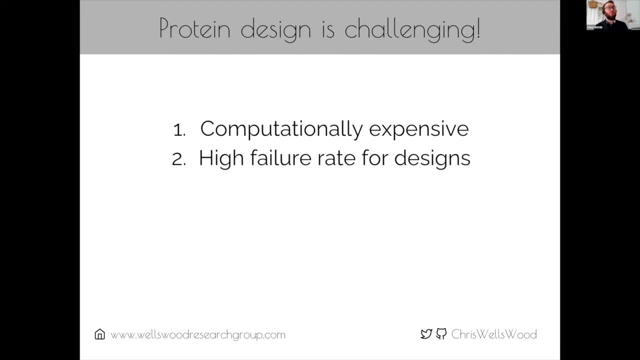 in the world when they're applying these protein design, computational protein design algorithms, a large scale, it there's still a very high failure rate. very often it's around 90% of the designs that you there are look good on the computer, in fact, that you can't tell the difference between. 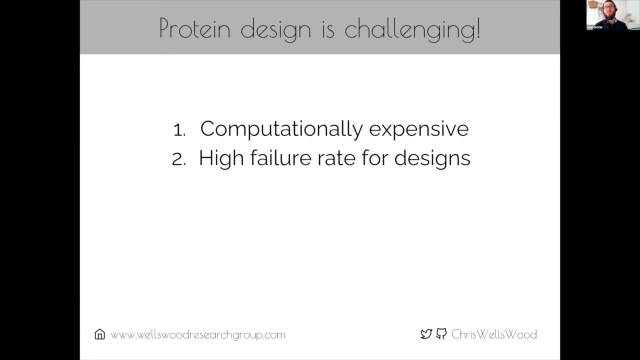 those designs, you take them into the lab And 90% of them feel for a variety of reasons. So some of them are insoluble and or the oligomizing ways, the unintended ways, or they're functionally inactive, depending on their 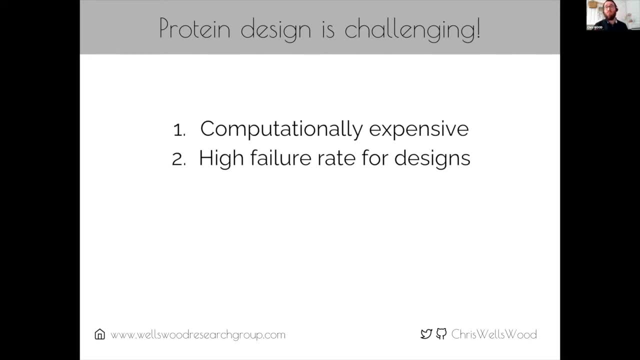 functions, So there's a high failure rate, And this is a huge barrier to entry, because it means that the number of designs that you're testing is going to be wasteful right without the resources you have. So this limits the kinds of people who 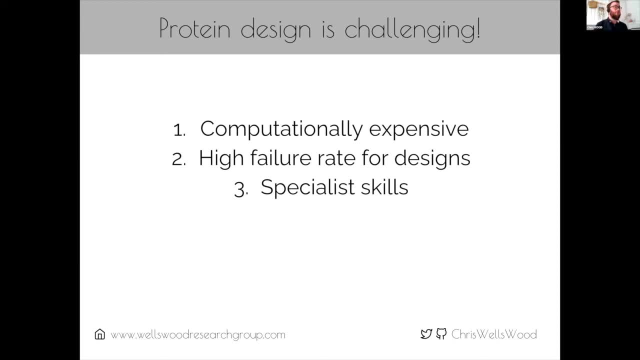 can apply. It also requires a lot of very special skills. So computational analysis, maybe molecular simulation, are a lot of things. So if you're a molecular biologist or something, if you're thinking about approaches to solving a problem, protein science probably not going to be the 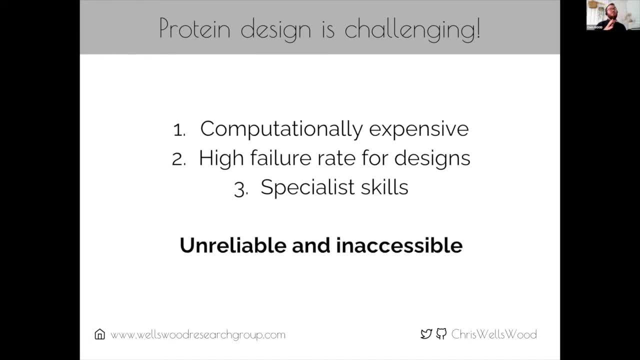 first thing on your list. So all of these things, I think contributes and other things contribute towards working, sending in excess, inaccessible and unreliable, And I think that we can address some of these, these problems, in order to get some, some easy wins. So how is my lab addressing this? Well, 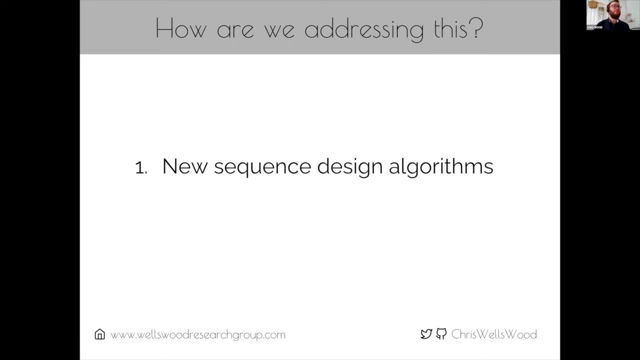 um. first of all, we're generating new sequence design algorithms, algorithms which are computationally efficient and incorporate lots of information, that make the designs more reliable, or that seems to be the case in the world. We're developing and testing these at. 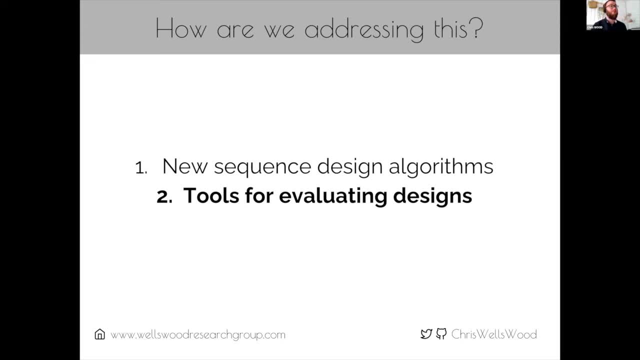 the moment We also are developing lots of tools for evaluating working designs And we're interested in in also all stages of that really sort of specifying what it is that you want your protein design to do in order to be for purpose, which is a challenging in itself and then a way of trying. 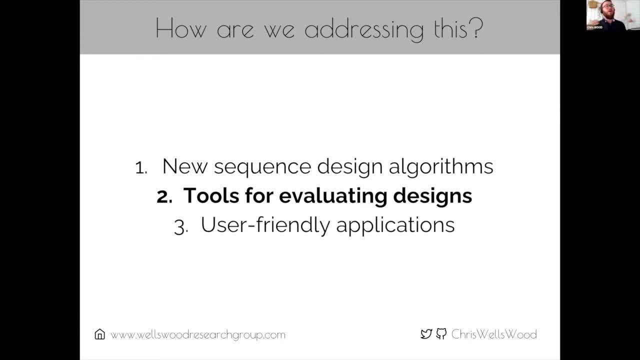 to get your proteins to see if it has this property. And then- and I'm going to focus on talking about that point too- And then as well, user friendly applications. I'll talk about that a little bit more. So we want to make them as accessible. 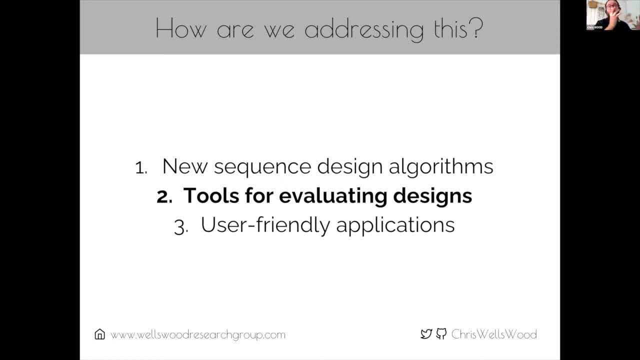 as possible. So whilst there's the sort of hardline, hard hardcore command line applications that people can apply a scale or on HPC, we also have user friendly web applications that can do maybe 80 or 90% of maybe 20% of the. 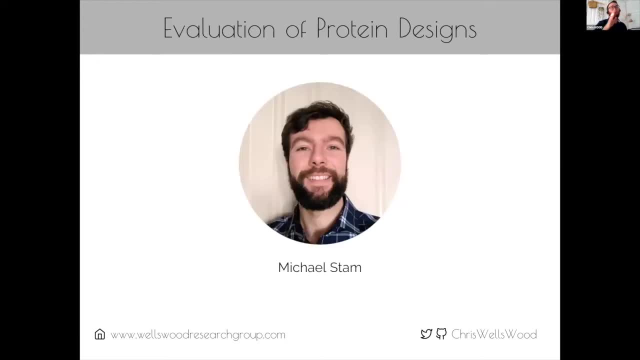 covers 90% of the use case. Okay, so the work I'm going to talk about here just a little tiny bit of the work that goes on in my group, And it was mostly done by Michael Stam here. So, as I've mentioned already, most design proteins. 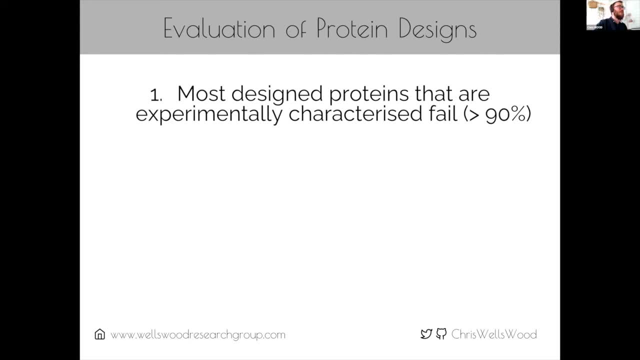 are experimentally characterised to be classless failures for a variety of reasons. Another very interesting thing is that there's a good body of literature that's saying that it's actually very difficult to distinguish good designs from bad designs. So, for example, in a paper from a manually patches. 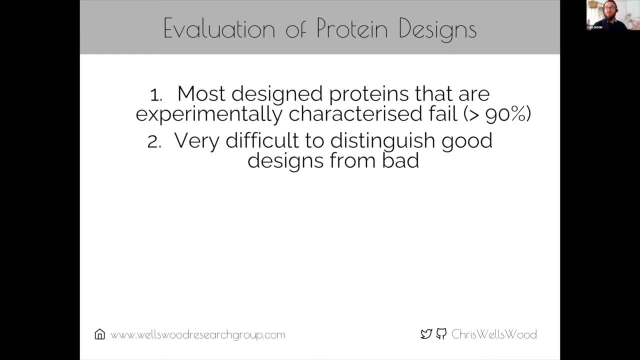 group in Leeds. they looked at trying to evaluate Rosetta designs and they had. they had confirmations. So they had confirmations for one design and they looked at the top 100 models which they couldn't tell apart from the Rosetta scores And it wasn't. 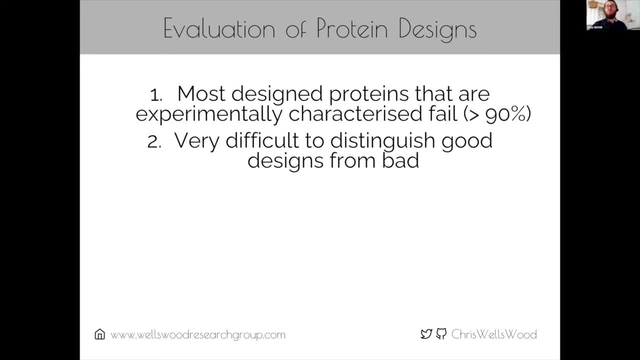 it's not like the number one design- the best ranked one was- was the successful confirmation that was adopted. It's very hard to distinguish those designs apart, So this is something we're interested in. Another thing is that I've kind of mentioned already. 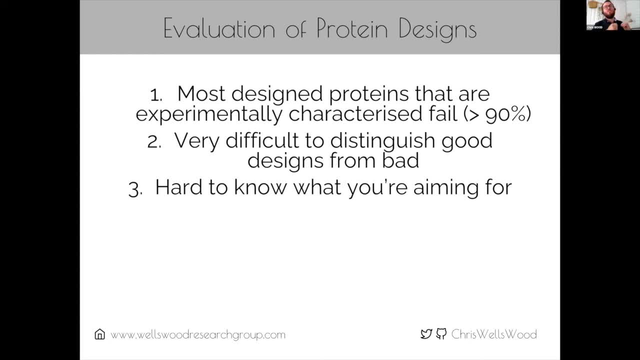 is that the objectification problem is quite difficult. How do you say what it is? what properties should your protein have to be for purpose? So you, if you're you're thinking maybe about catalysis or some, or you know, a structural 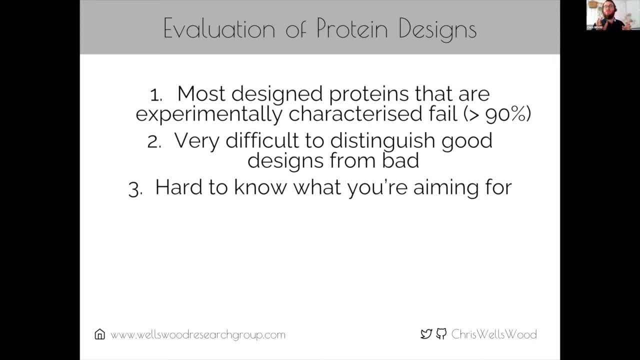 protein or something like this. you can think about this, this end usage, but you've got to consider all sorts of things, of course, to start with the. you know the DNA construct and how that's going to be translated in the environment. 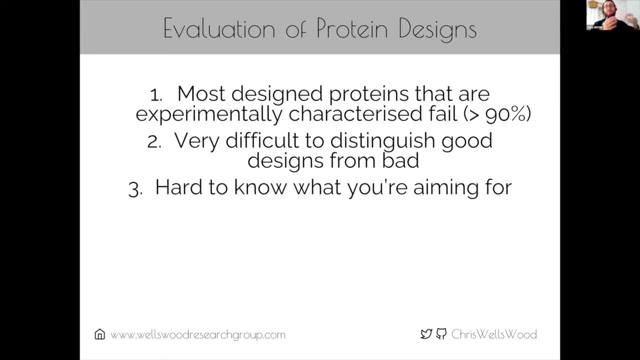 and transcribed and translated in the environment you're working in. But how is that going to be trafficked, How's it going to fold, and all of these things. There are things that you need to consider. So there's lots and lots of properties and, as well as you know, properties like 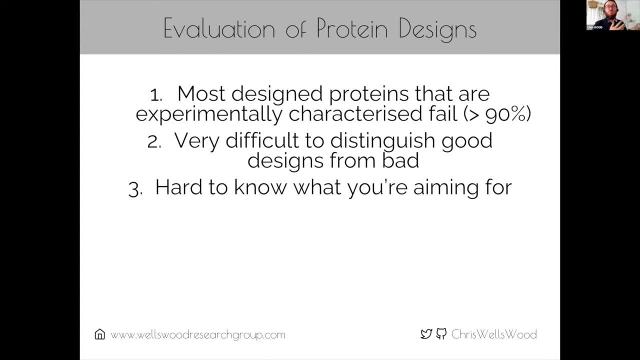 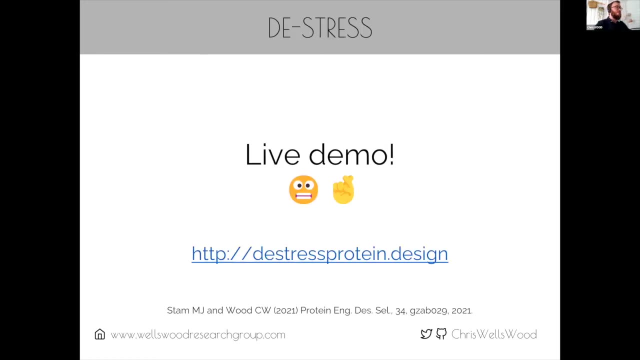 the ones that David were mentioning: thermal stability, for example. maybe your protein would be useless if it didn't work at a particular pH range or temperature range. So we developed a destress, which stands for design structure evaluation services, to tackle these, these challenges. So I'll 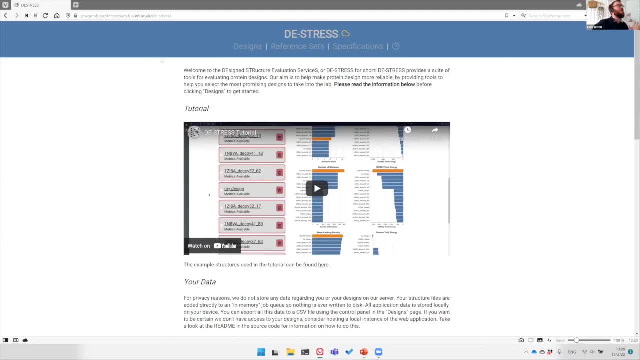 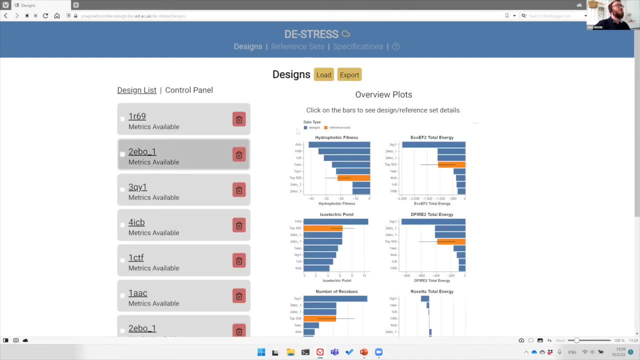 do a little demo of this here and hopefully we'll go okay, So you can go to that web link that was there, destressproteindesign, And you'll go to this web page. And how it works essentially is that you upload some designs that you've generated through. 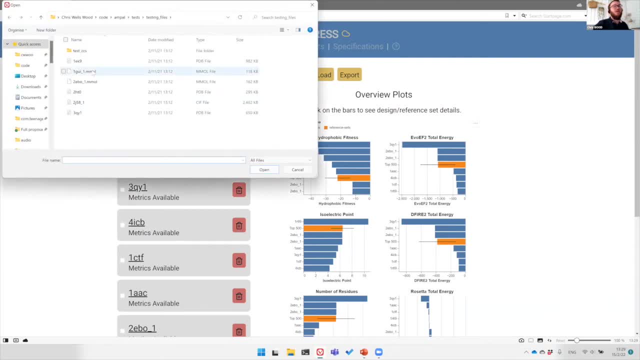 whatever program. So this could be Rosetta or anything, just their PDB format models at the moment it'll accept. So let's just actually you can load them up and they'll go off to our server and they'll run and calculate a whole bunch of. 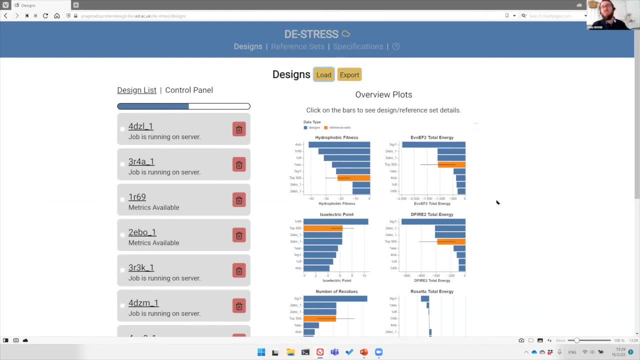 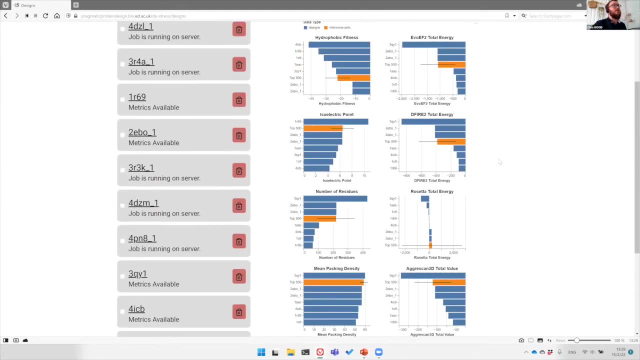 metrics for them And you can see that I've pre calculated some metrics. These are just using existing PDB structures for the protein data bank And you can see that it calculates all sorts of different parameters and new ones are getting loaded in as they're finished there, And there's there's all sorts of 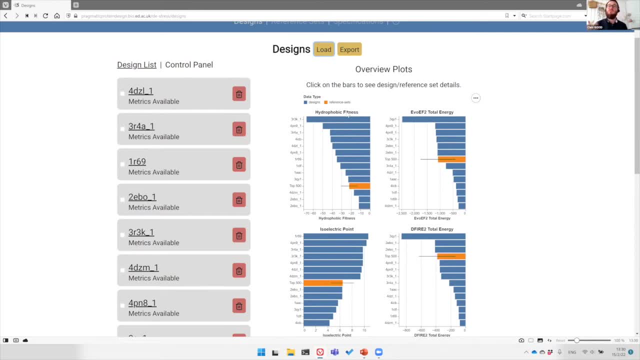 things. So hydrophobic fitness. these are either existing algorithms that we've implemented or using existing software to run these things, And it's a big meta scoring approach that we're taking. So statistical potentials: all atom force fields measuring hydrophobic fitness. 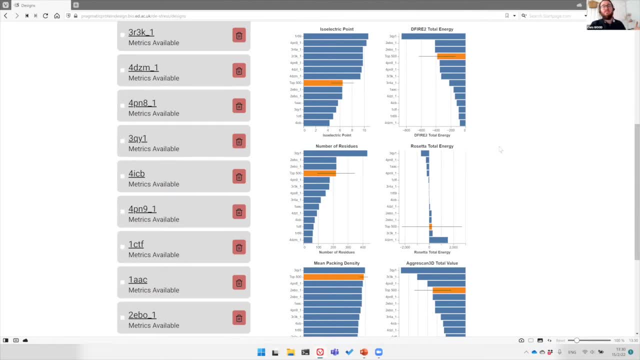 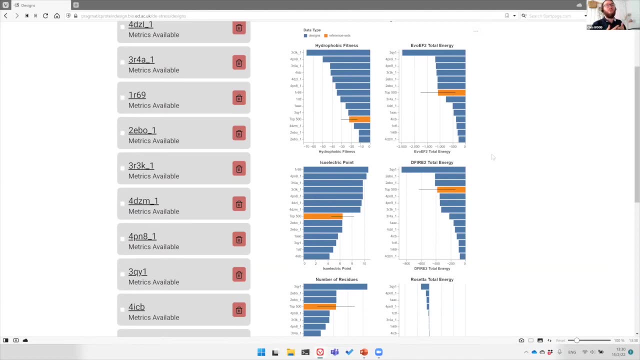 measures of quality, of packing, aggregation, propensities, And the idea, in the first instance, is that we're not telling you which designs are good or bad, we're just telling you as much information as possible about your individual designs And you can, you know, click on one of these here and go in and find a. 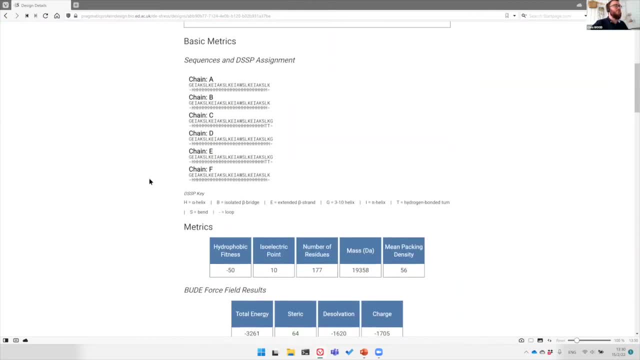 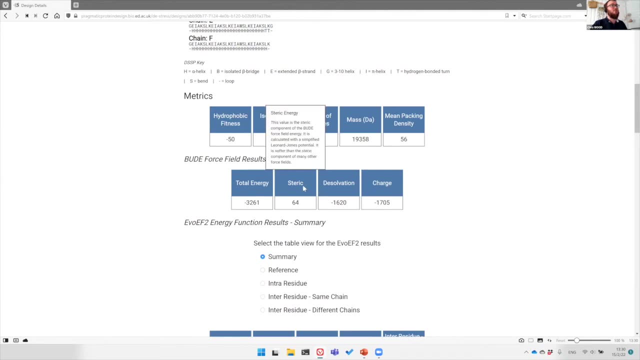 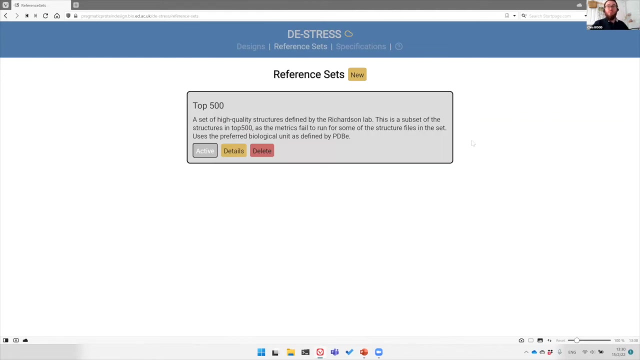 bit more information about the particular protein and its sequence, and then all these parameters And then, for all of the all atom scoring functions, for example, you have each of the individual components. you can see this. we also have this um called reference sets, And this is a set of known protein. 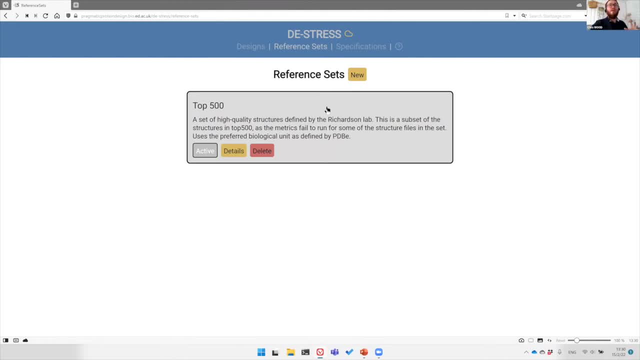 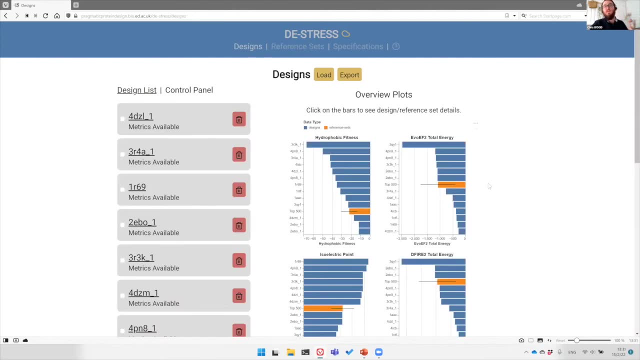 structures- or they can be models that you've uploaded as well- And it calculates all of the metrics for these models and generates a sort of aggregated pool And you can use this as a basis to compare your designs to. So, for example, 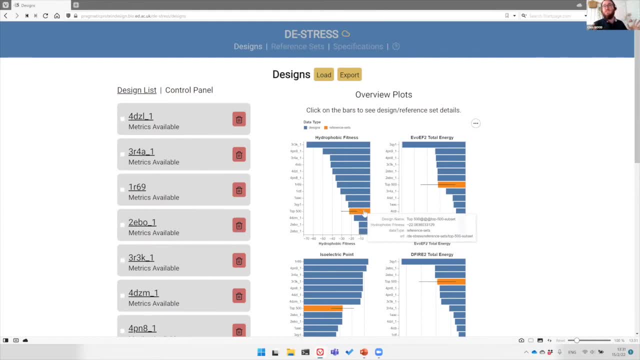 we've got top 500 here, which is a set of sort of high quality crystal structures which were came out the Richardson lab a couple of decades ago. So you can see here you can have those structures compared to your designs, For example. we can see here that you know that what. 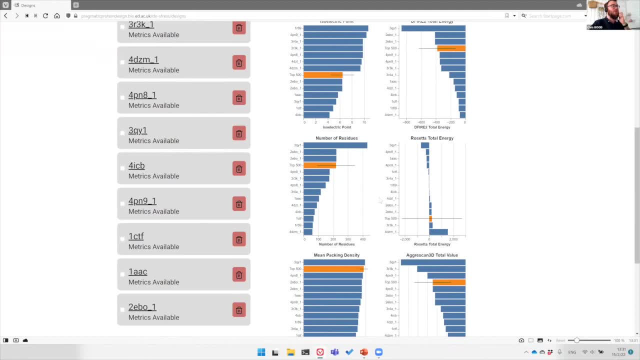 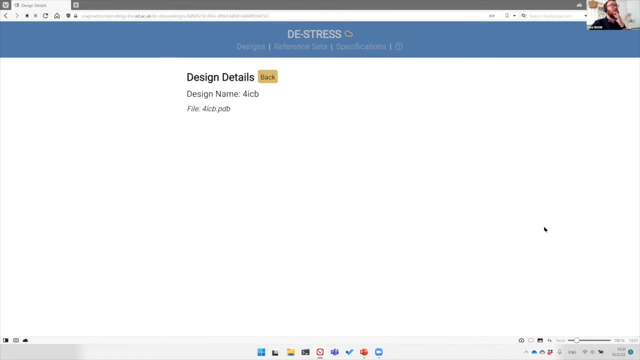 the, if we F rank is, or the fire score and the size of them, all sorts of things, And in fact, if we go back in and pick one of these, then we we can get a bit more detailed information about how your particular design relates to this, for example. 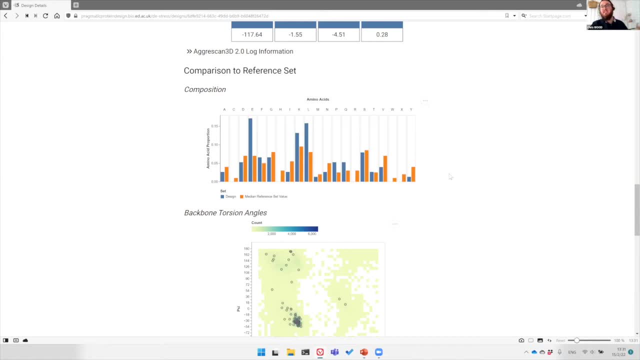 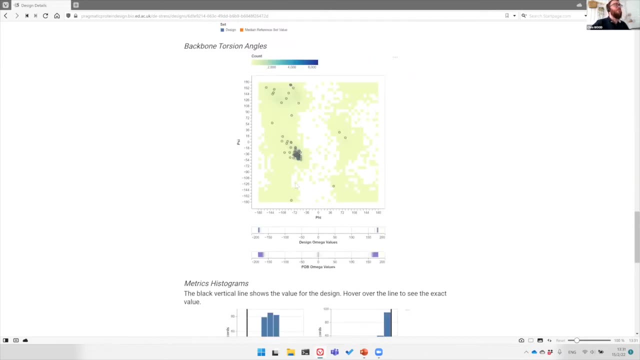 looking at the relative composition so you might be able to get an idea of the metabolic burden of your protein. if it's poly tryptophan, maybe it's, it's going to be difficult to express, or something like that. So you can see, here you've got the structural space. 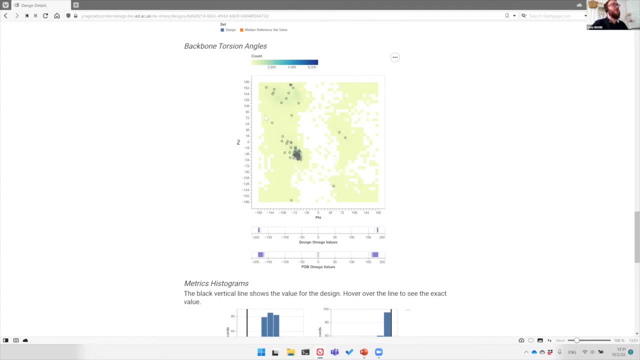 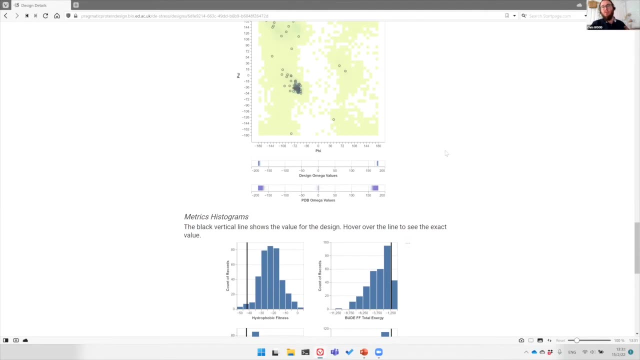 that's, that's occupied by the reference set which is in the background here. So this 2d histogram and then you've got the your individual amino acids of your design there. So you can see: is it going into the right region of structural space or? 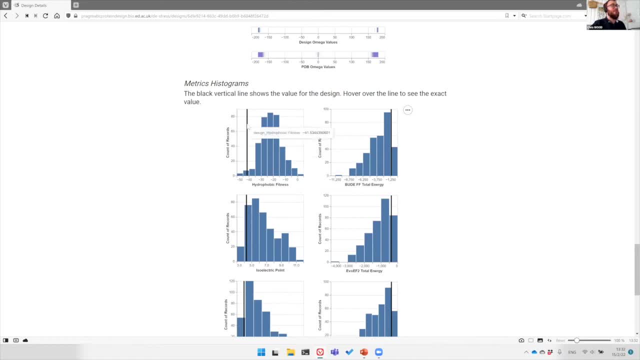 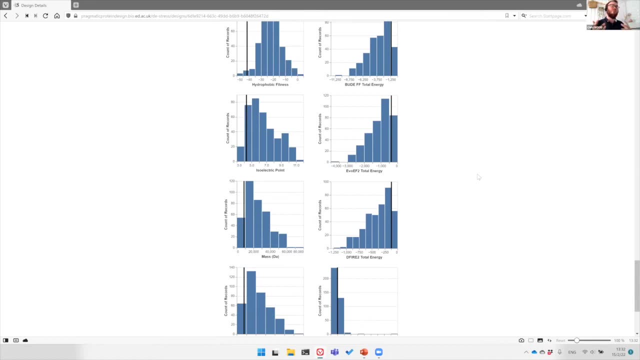 the region that you're expecting, And then you can compare the distribution of your designs, of your design, in this black bar to the distribution of the reference set. So you can start to try it. it's hard to determine what properties your protein should have, So it's useful to do this comparison to be able to 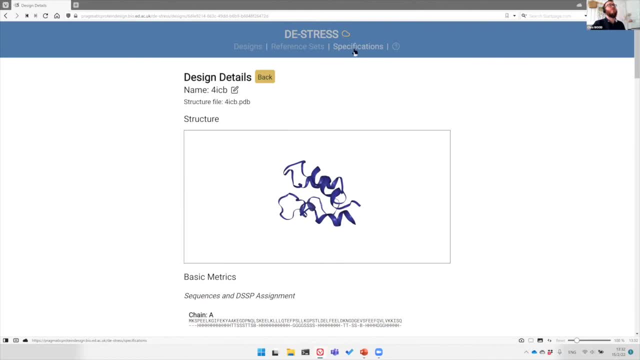 see if it's like a, if it's likely to be fit for purpose, And the final thing is specifications we're not going to get into, and this is a formal way of describing the properties your protein should, should have, And you can apply this to evaluate your designs Now, like 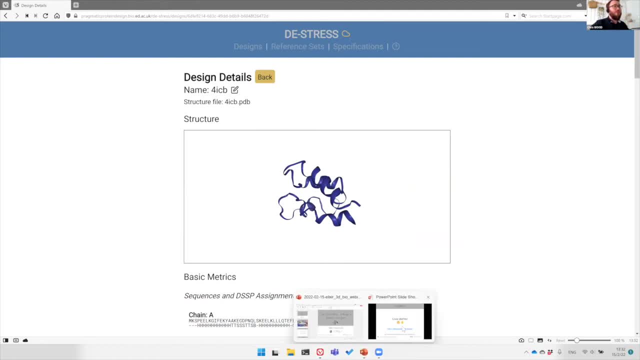 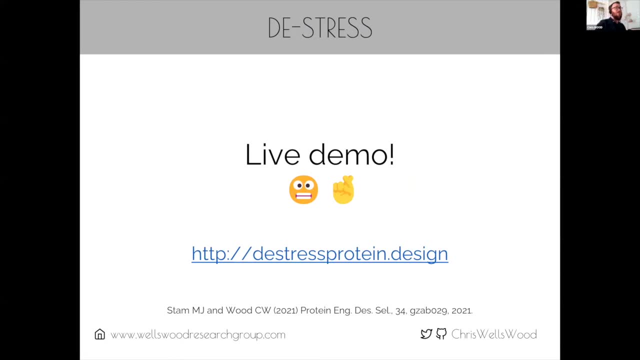 I said you've got this accessible web application but it's also, you know, available on the command line into. it's easy to deploy and local compute So you can run this at scale. And then I want to show you that you know it's not. 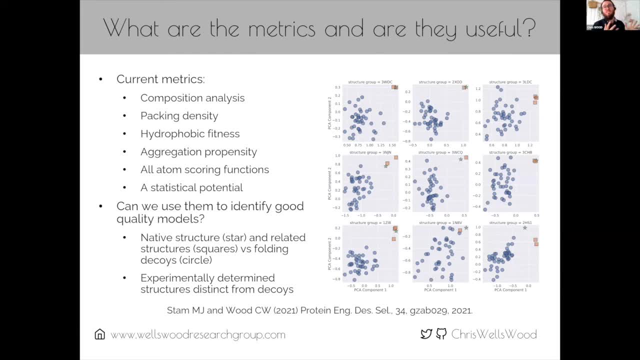 hopefully demonstrate to you that this is. it's likely that this is going to be useful. The metrics: we've included our standards, like the result, of course, in computational protein design, so we know that it's useful for design right, But we're hopefully I can show you. 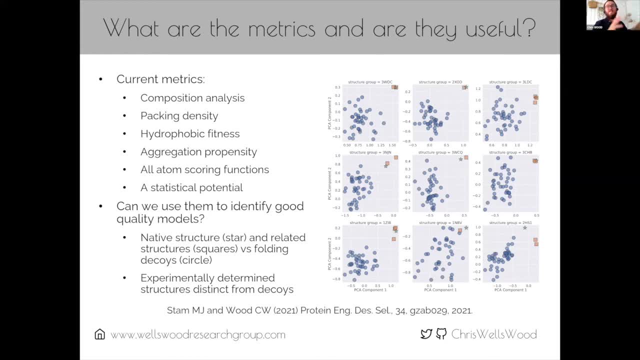 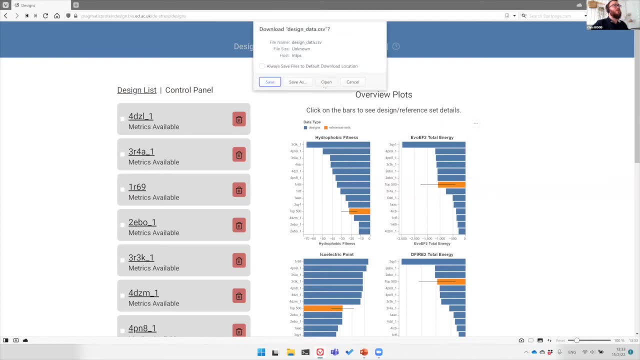 that you know we've got an indication that it's useful And when you can mix together lots of different elements. One thing I didn't mention, sorry- is that if we go back here we can export that, all the data from this, so you can go and 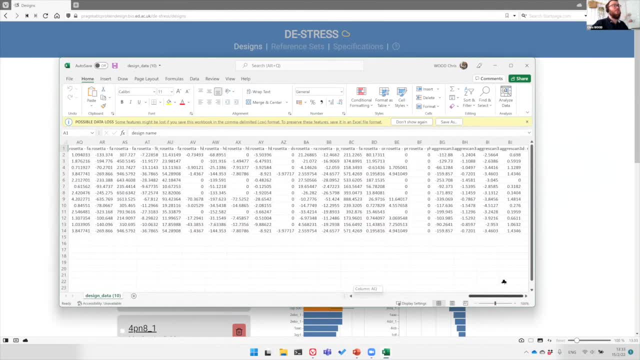 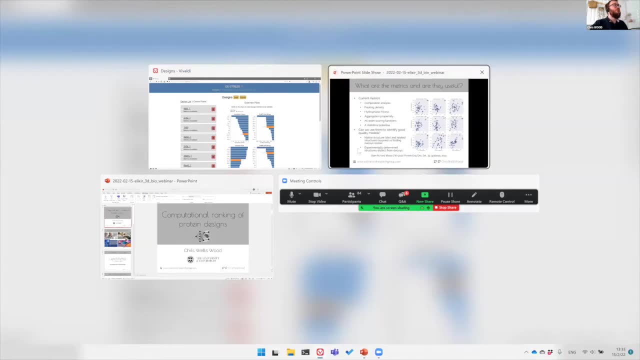 interpret it and do statistical analysis on anything that you'd like to do. And it includes actually all of the component scores For each of these different force fields and whatnot. So when we go and look what we wanted to try and when we're 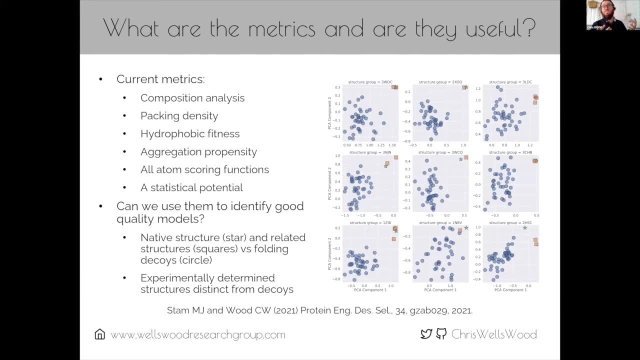 publishing it. we wanted to say: look, this is useful, we can use it to distinguish good designs. And in order to test this, we compared it from. we looked at folding decoys. Now, these are structures that have been generated to trick folding. 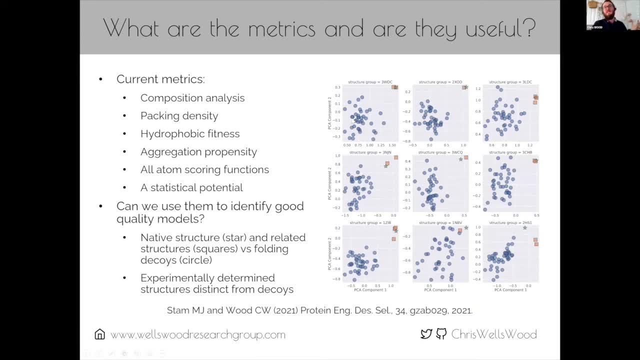 algorithms to test them, And we looked at this one, that's this set that was generated by a program called 3d robot, robot that comes out of the Zhang lab, And these the star. the star is the structure of the decoys, And then the decoys are. they're. 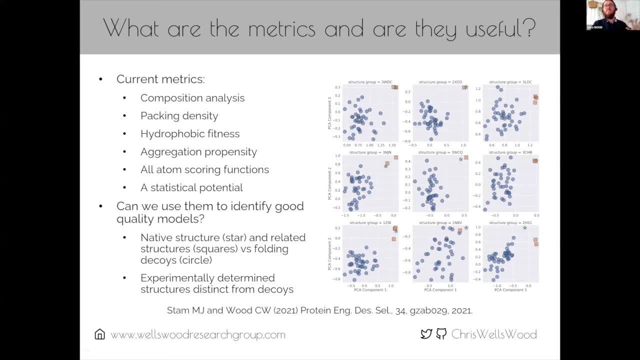 the known structure. And then the decoys are well, well packed at non trivially identifiable structures, structures that are not the thermodynamic minimum, or at least what the structure is. And as well, in squares here we've got other structures of the protein or closely related proteins to compare. to compare. 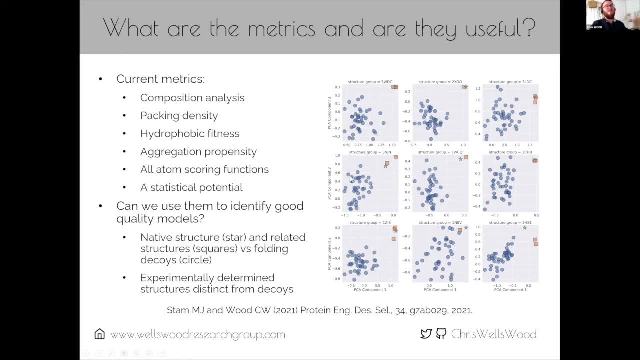 the level of variability. And you can see here that we perform principal component analysis on a selection of the metrics a and then we can identify that the, the folding decoys, cluster together in a space, whereas the known structures, the experimentally determined structures, are up always in this. 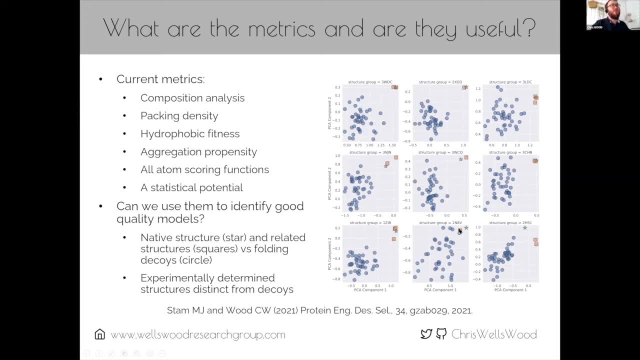 this upper right hand corner, separate from this, this main cluster. some of them are more distinct than others, But it is from this point it's trivial to identify these, for example, so you could use this to say: well, how sort of, how likely is it? 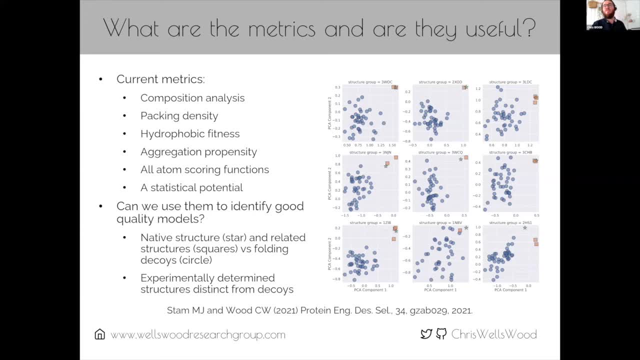 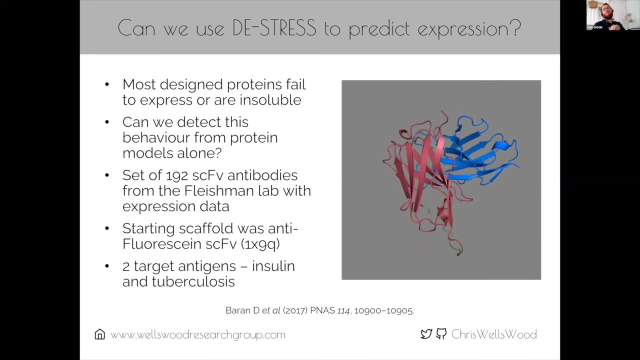 that this design I've got, how good is this model that I've got? How much does it look like a known structure? So let me do this work for 90 feet structures. So now we're moving on. we're interested in antibody design. 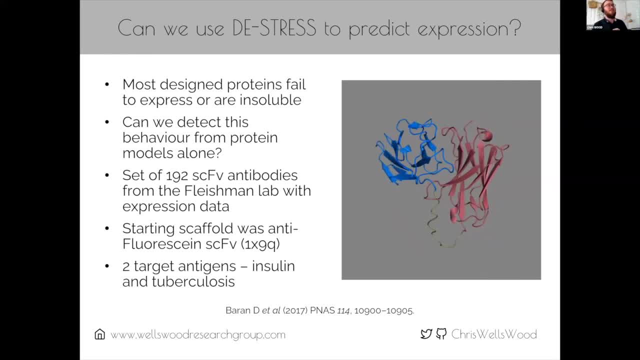 and can we use the these types of metrics to identify high quality? This is a engineering, especially in the final stages of generating antibody based therapeutics. Very often, what you want to do is to point mutations to your binder that you've identified through a high throughput screen, And we've 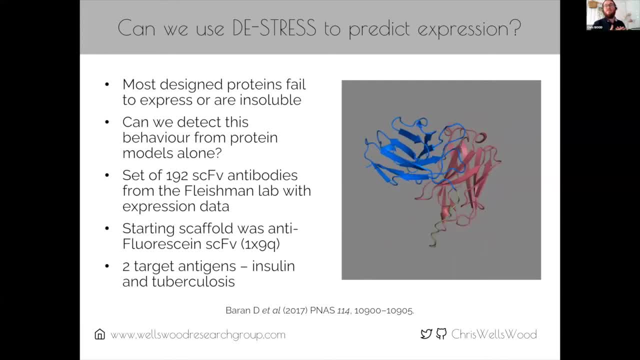 been talking to a bunch of companies about this And very often there's a high failure rate on just generating those point mutations. So a single point mutation will lead it to misfolding or the massive reduction in in the production levels that you can get, for example. So identifying this, 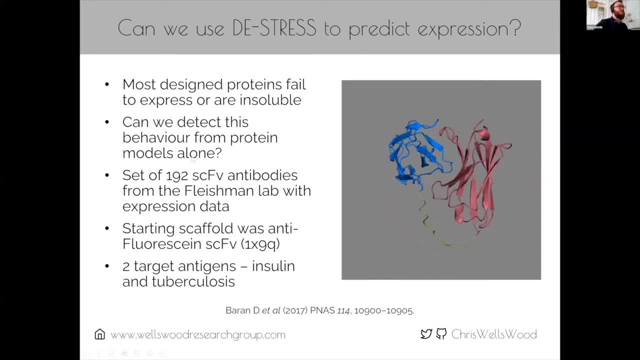 early on is very useful, And one thing that we're looking at is single chain antibodies And we there's a lovely data set from the Fleischmann lab in Weissman in Israel. They have multiple design rounds of generating single chain antibodies And 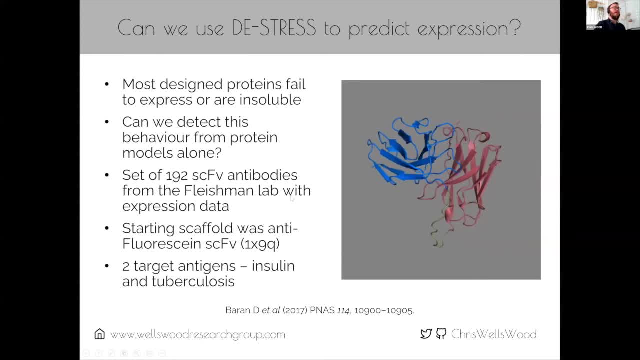 it was starting with a scaffold for antifluorescein, And they optimized it in five design rounds in order to improve it. So this is how they look. you've got the light and the heavy chain and they're joined together with this with a long 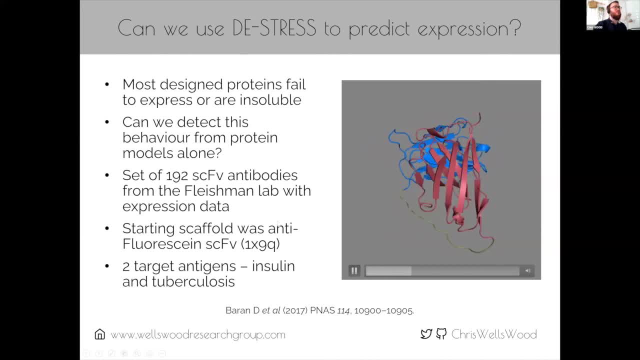 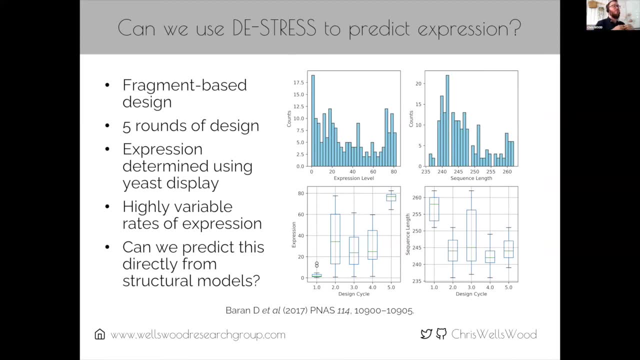 linker here And this is a structural prediction from half of old. So initially Michael did some analysis of this data set to try and look to see, you know kind of, how the designs varied from one another, whether we serve systematic variation. 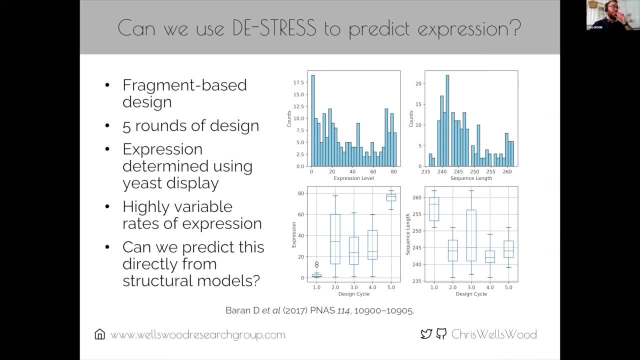 And you can see here that they had a measure of expression level, which is what the first thing that we were looking at: to see if we could detect, so that you could exclude ones that are likely to have low expression and never make those ones to start with at all and save yourself a whole bunch of 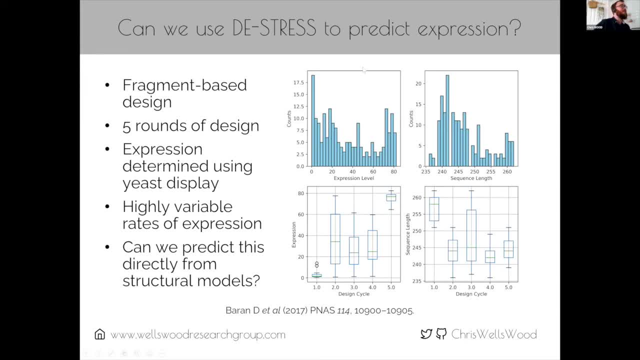 money on DNA synthesis or get more designs that are likely to be successful. So they were determining expression levels using yeast display. So protease resistance with yeast display. I think that's the method that they were using And you can see there's an expression level that goes from zero to 80.. 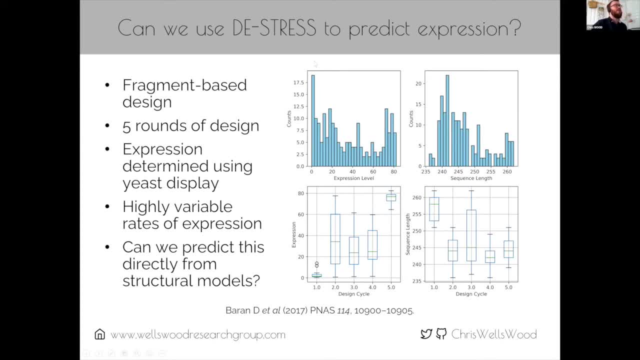 80% of the of the maximum fluorescence And it's not normally distributed. you've got a lot of low expression, you've got sort of peak for high expression and then a lot of stuff that's in between. And if you look at the expression, 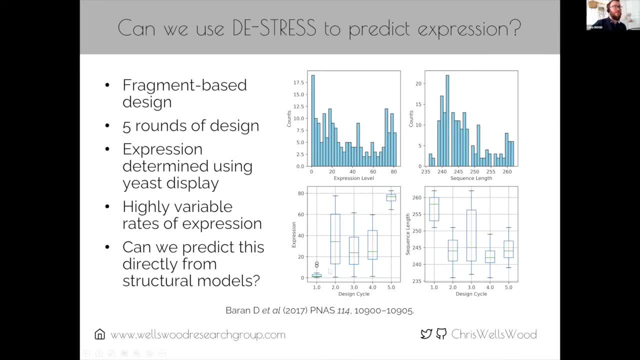 across the design runs. you've got the first round of designs had very low expression and then the last one had very high and in between it's sort of quite interesting- got large variable sort of ranges there And as well they're just to. 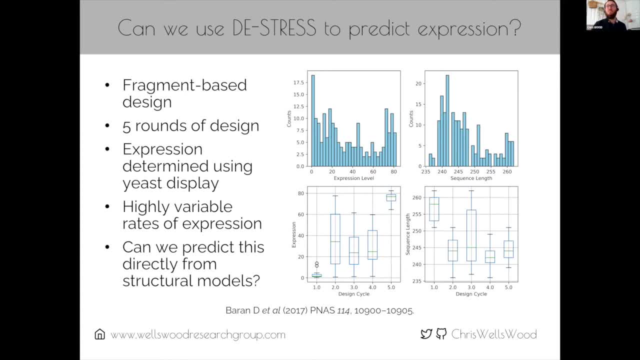 point out that there is variation in the sequence length as well. So they changed the linker and the change loops and whatnot, because they were doing fragment piece. So what we are interested in is: can we, can we, you know, generate structural models for? 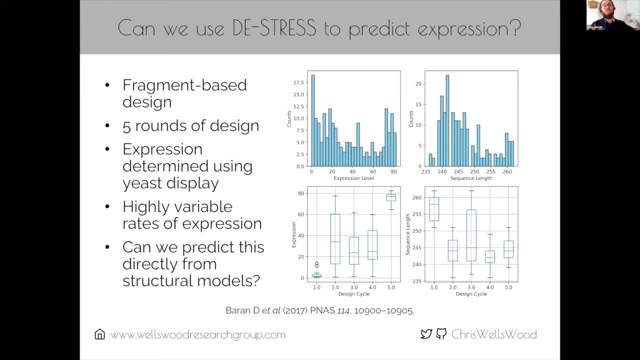 these, run them through- which is the stage you'd be at once you've done the protein design- and then run these through de-stress to generate some structural metrics to determine whether these are good designs or bad designs. And this is, this is this was the result We- yeah, like I said, we generated. 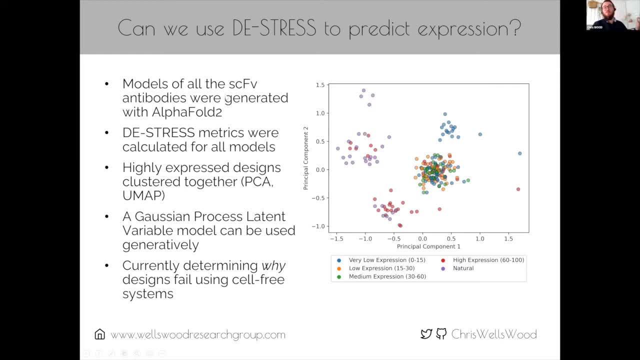 them with alpha fold And we calculated all these metrics and we did principal component analysis as well as some other clustering techniques such as you map, and showed very similar results. And you can see here that there's. you get clusters of low expression. sorry, two seconds on this filter So I can see. 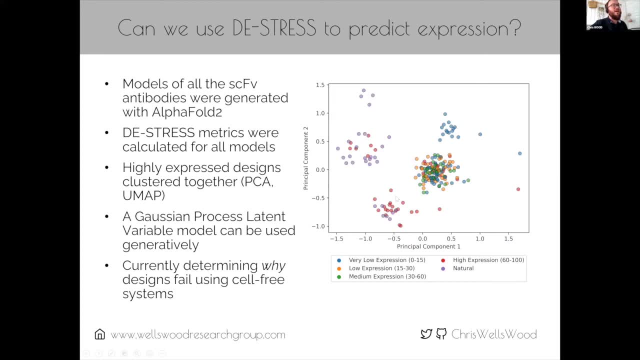 cluster of low expression over here And then you can see the high expressions in two separate clusters and then the low to medium expressions all clustered together in the middle here. And what's really interesting is if you, if you go out and get other known structures of 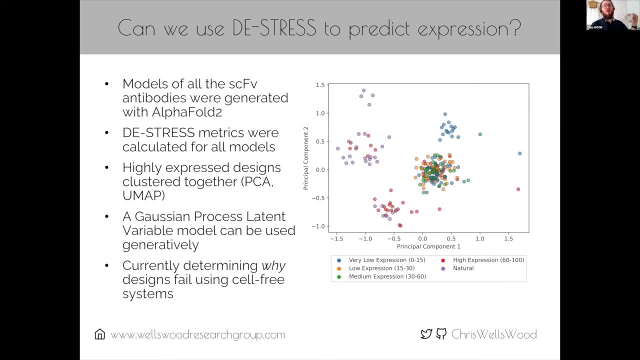 single chain antibodies then, which are totally different targets, different, very different sequences, and then you compare them to this and they're under this natural. so natural is maybe the wrong word to use here about known structures. If you calculate the metrics and compare them to these, they 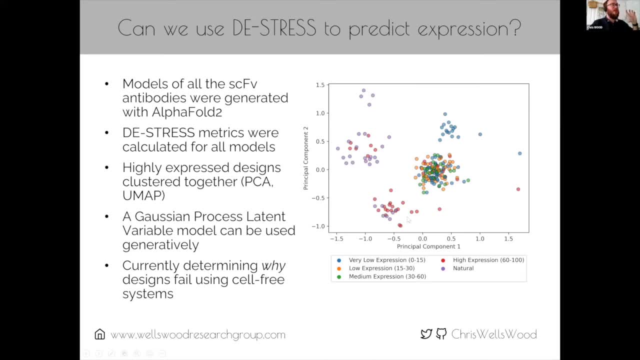 cluster together with the high expressing structure. So there's some information in the, in the metrics that have been calculated by de-stress, that indicate that these ones are, these designs are going to be high expressing. Now we're looking at some of the things that we're looking at the moment. 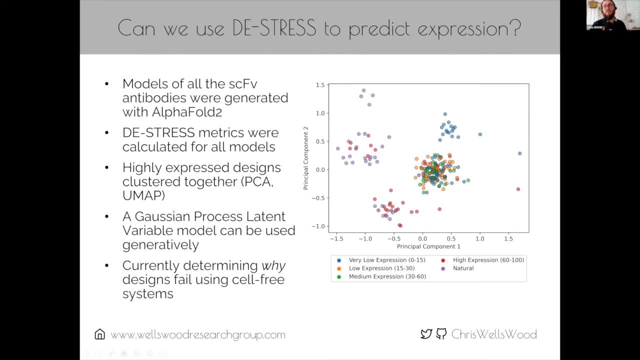 in the in the lab, for example, we're using cell free to try and determine why they failed, So we can get a bit more information about what's going on, because it's very interesting. The sequences are very similar, but some of them are very low. 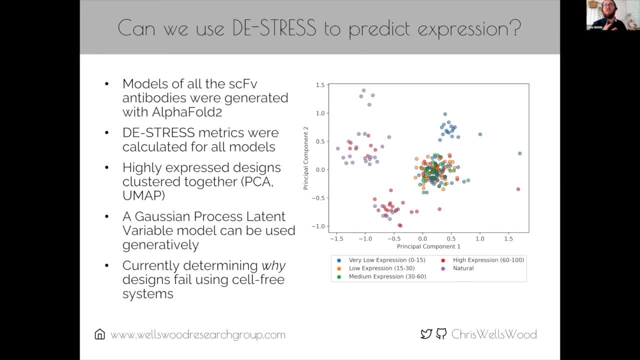 expression. some of them are high, and we're trying to determine if we can figure out what is this going wrong, So we can change methodology, for example, to account for that. Another thing that we're doing is that, as well as using PECANUMAP- 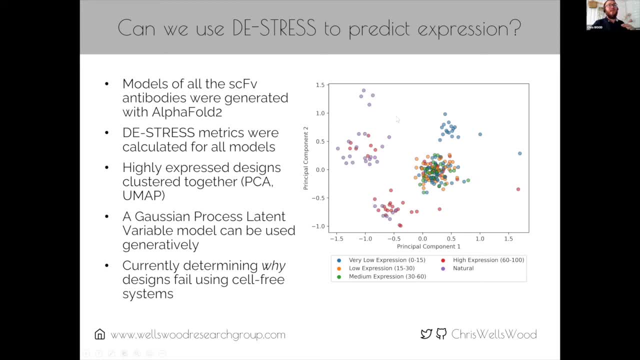 we're using something called Gaussian Process- Latent Variable Models- in order to be able to sample from a latent space and identify new sequences that are close together with the higher expressing sequences in structural space, or identify if our designs would fall into those regions and use it. 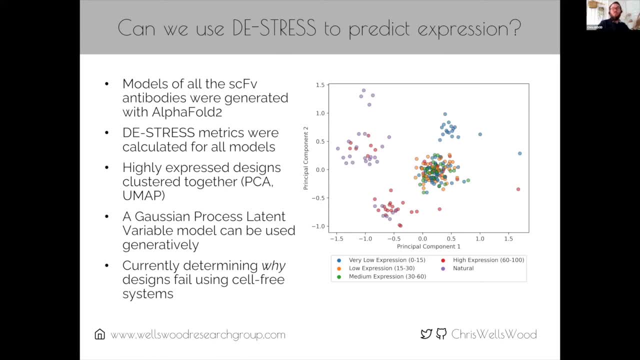 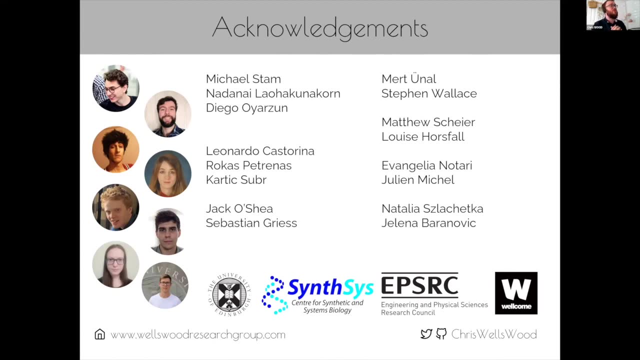 generatively so that we can do design. Okay, so that's just one little aspect of the work that goes on in the lab, but lots of other stuff as well, And Michael Stamm, my student, did most of this work and he's co-supervised by Ned and I and Diego as well. 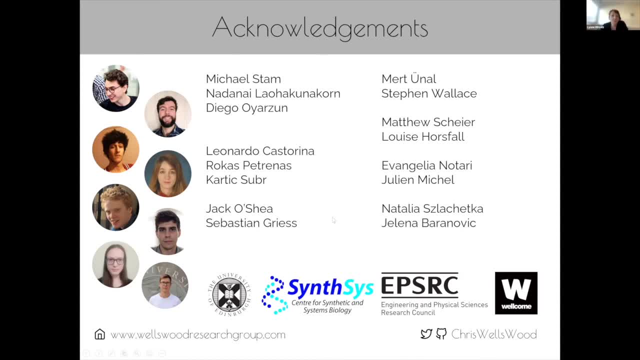 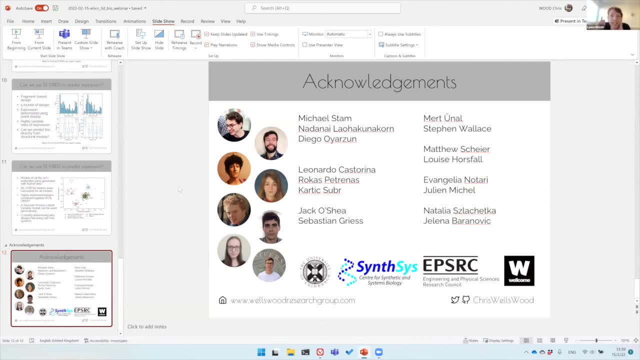 So thanks very much, Great thank you very much. We have not really time for questions, but I'll ask you one question myself, which is: have you ever analysed NMR, determined structures? Have you ever run rather than like a 3D robot? 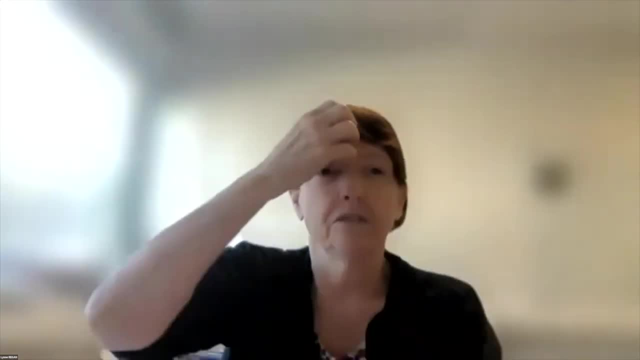 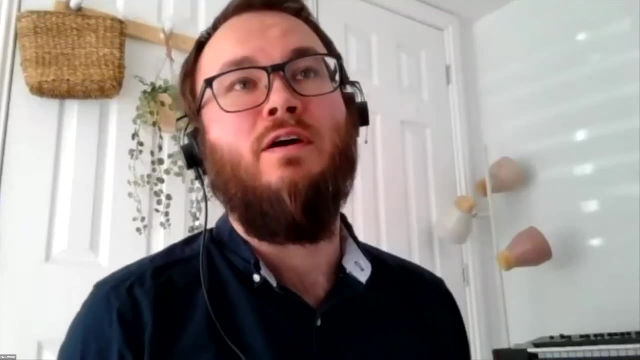 decoy, have you ever looked at any structures determined by NMR? No, no, we've not. That's a really good. that's a really good point. We've kind of avoided it, necessarily, but we've not looked at them. particularly We have for lots of our design-based 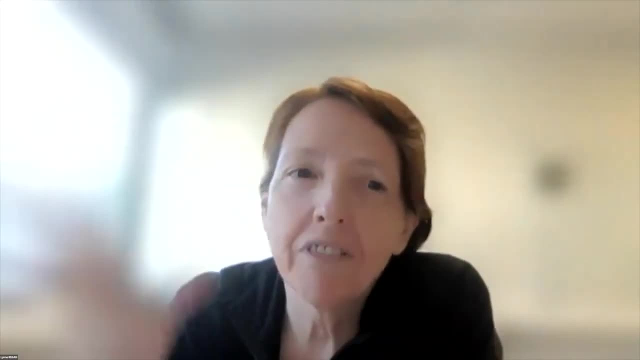 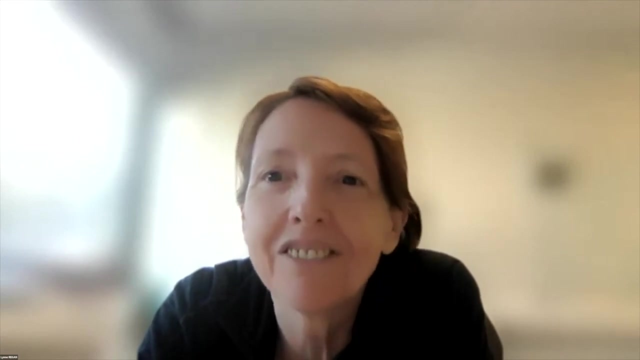 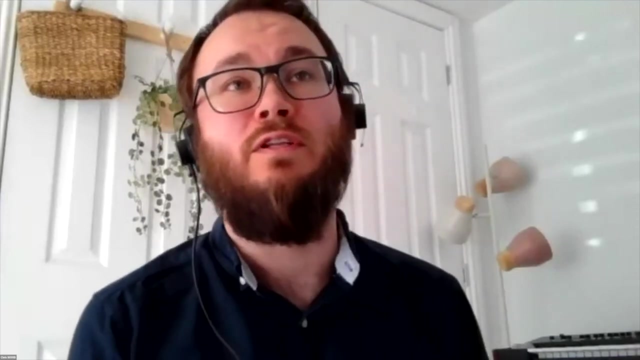 algorithms. and I asked that because in recent work we found they look a lot like unsuccessful casp things, So I was just wondering how they work. Yeah well, this is interesting because with our design algorithms, our sequence design algorithms, the quality of the 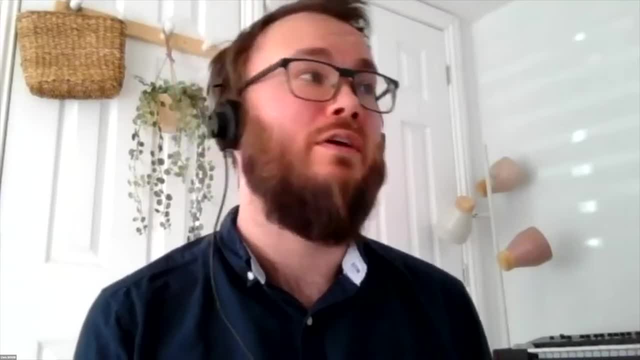 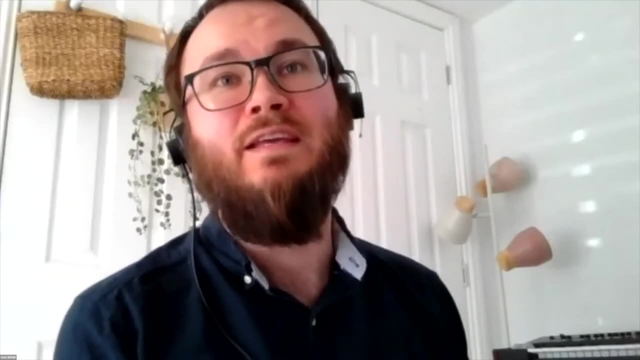 structural prediction. the sequence predictions are much lower than on extra crystal structures, which is not so surprising. You see this with AlphaFold as well. Yeah, it's trained on crystal structures And I suppose it depends what we're aiming for. We're aiming for. 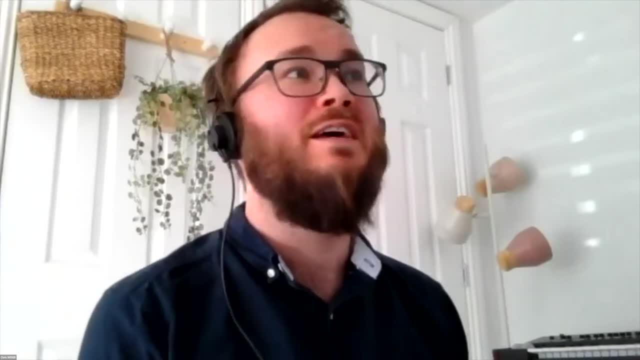 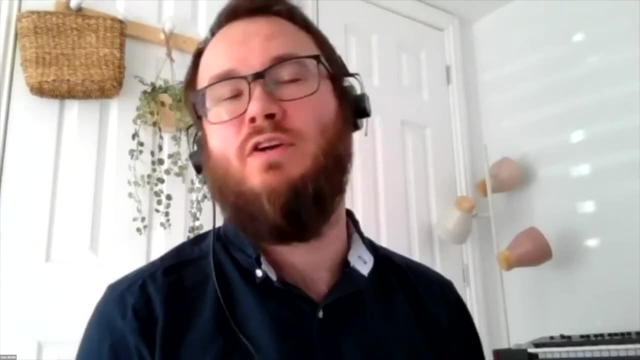 things we can crystallise and publish, So it's maybe not too much of a worry for us, But really, yeah, I think it would be better to identify, you know, soluble- sorry at room temperature and whatnot- and a solution based. 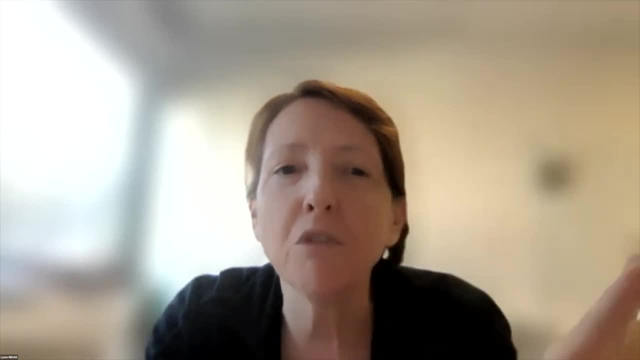 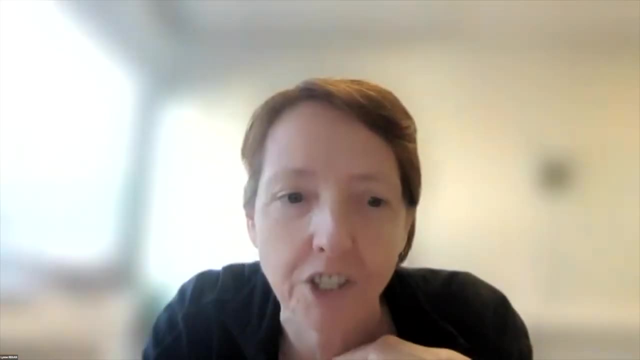 Yeah, though I don't actually. well, we'll move on. we can bring this into the discussion. Thank you very much. We're going to save some of these questions for the final discussion because I don't want us to be too rushed. 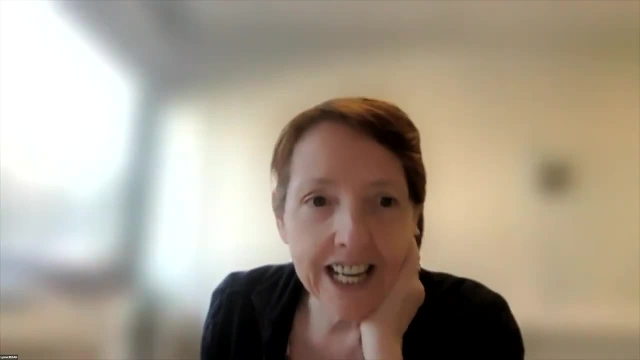 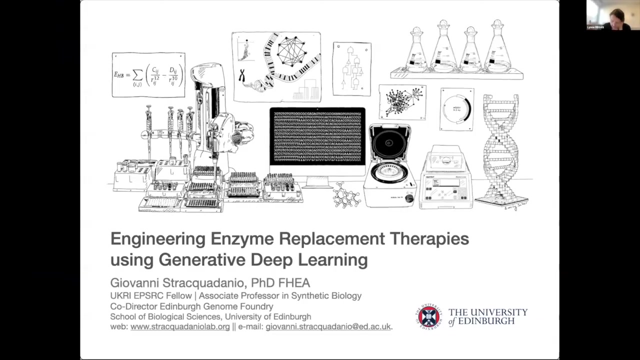 I want to move over to Giovanni now, And he's going to tell us about using deep learning to do design on what I would call a practical target for enzyme replacement therapies, And so this is like. okay, we've said in the past, we want to learn. 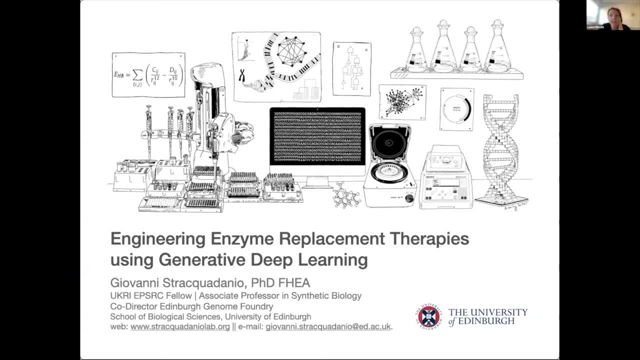 about how proteins work, which we're still doing, But here is an application of design methods towards a target that could actually be given to people as a replacement. So, Giovanni, take it away. Thank you very much for the kind invitation. really a pleasure. 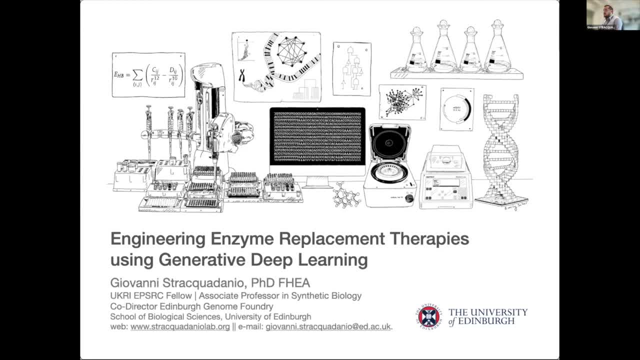 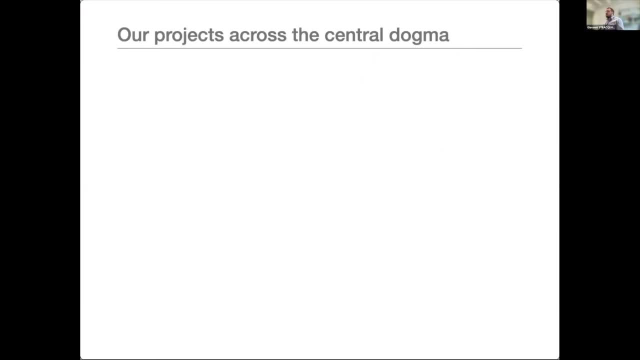 to be here presenting some of the very recent work that we have been doing in my lab, which actually it's working across all the central dogma. I should say we're really interested in genomics, to begin with and specifically understanding irritable components of cancer, but also we build genomes. we 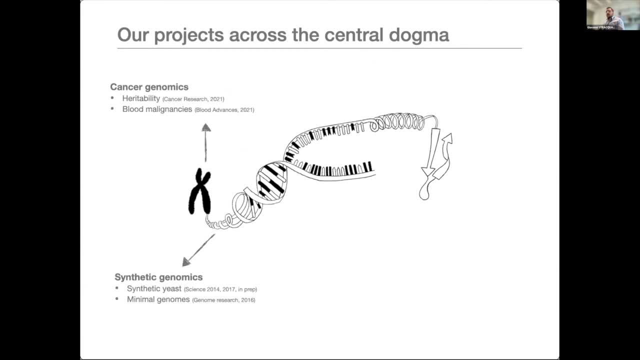 are part of the synthetic yeast consortium And we have moved along the line. We're trying to understand the gene expression at the network level, both in disease and pathological states, And also we want to engineer expression by modulating the codon usage in. 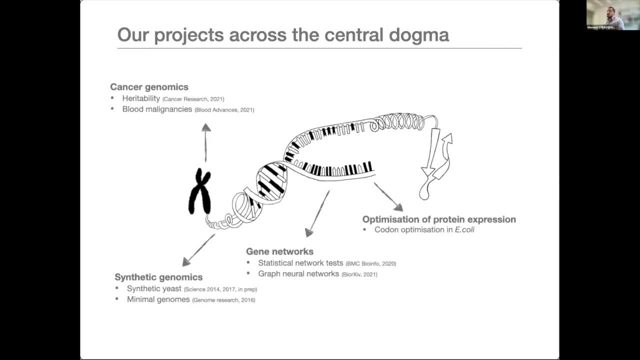 E coli for heterologous protein expressions, And the new projects we are really excited about is really trying to engineer better enzyme replacement therapies, And I'll talk to you through what we have been doing so far And, of course, this is not a really well-known project, but this is a very, very 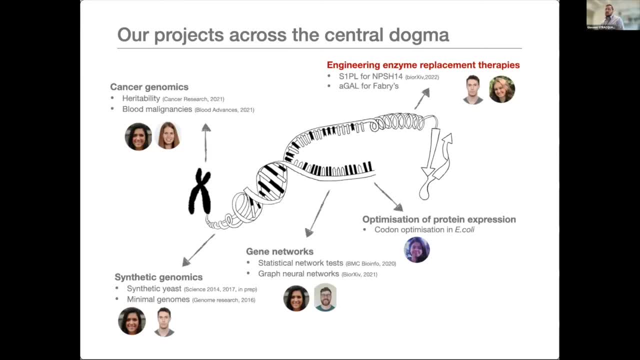 interesting project, not necessarily all my work, but it's actually the work of the amazing students in the lab who had taken all my ideas and made them real, and also the collaborators that are really making all this science possible. And if you see something that you like about replacement therapies and 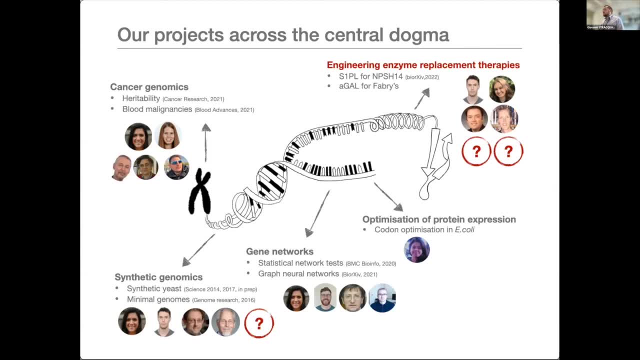 study genomics. we have three postdoc positions- two experimental and one computational- to start almost immediately. So please do feel free to get in touch by email. So today we're going to talk about genomic therapy, the genetic and genetic therapy, the genetic and genetic therapy. So today, 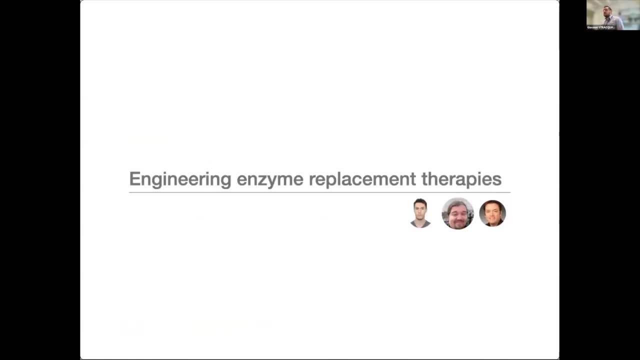 to talk about engineering enzyme replacement therapies. As I said, this is really a work led by one of my PhD students, a very talented mathematician who actually embraces protein more now, Evgeny Leobzaev, and it's been a really great collaboration with Michael Herrera and 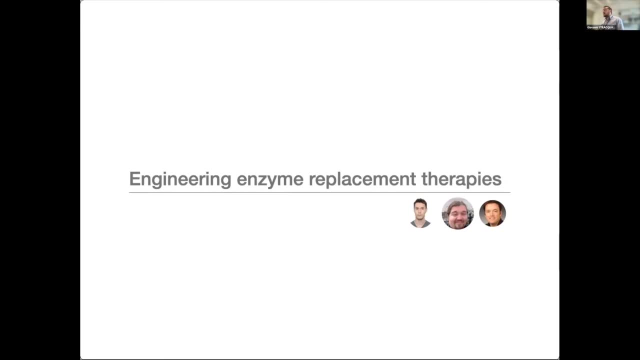 Dominic Campopiano, who are experts in biocatalysis, and we share a common interest in sphingolapids. So we all know that enzymes are proteins that catalyze almost every metabolic reaction required for cellular life, and the problem is that when you have an enzymatic deficiency, 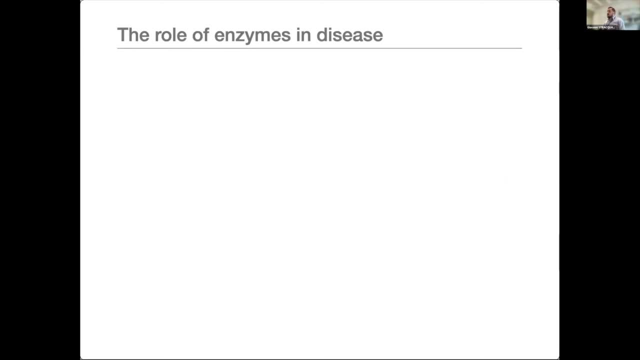 you get the accumulation of toxic level of substrate in the cells and you get very severe pathologies. So if you look at the cell you will see some of them are quite known, like Gaucher disease, Pompe and, a little bit less, Fabry disease, which we are really interested in. 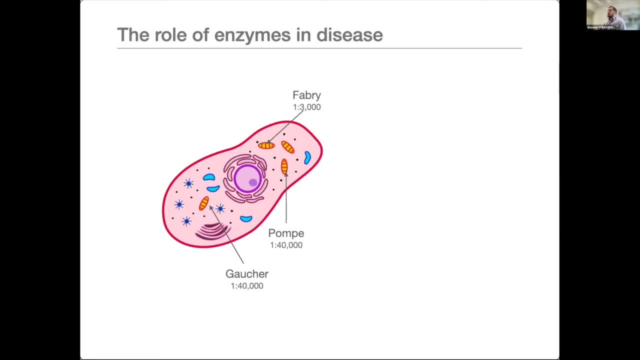 And the problem is that these diseases are very rare- usually affect one in 40,000 newborns, but the reality is that the spectrum of phenotypes that they encompass are so broad that the diagnosis happens very late usually, and so actually these numbers might be very much lower. The end game of 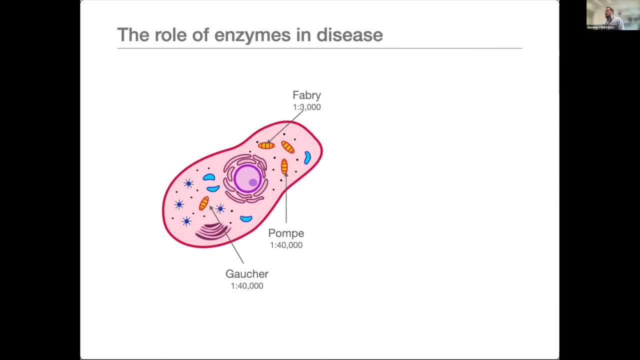 these diseases is that you have irreversible damage to specific organs. For example, for Fabry, typically this means impairing your kidney function, but almost all of them somehow impair heart function and some of them also CNS, which means that, at the end of the day, if you're 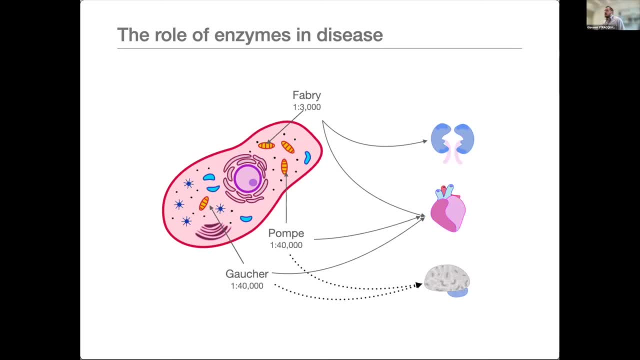 affected by one of these devastating diseases, your lifetime is usually very, very low. So how we are trying to treat these diseases. unfortunately, you cannot cure them, but you can improve the quality of life of patients and also increase patient survival by basically using replacement therapies, which is nothing more than. 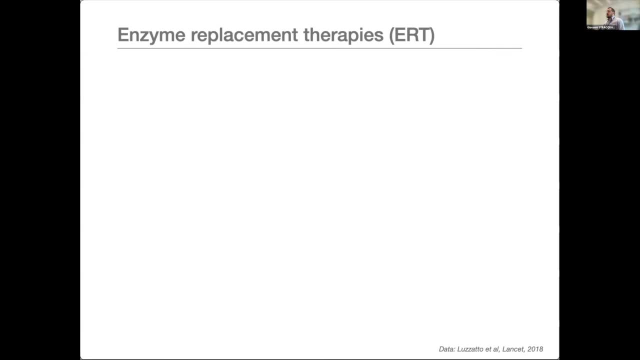 taking a recombinant version of the affected enzyme, do an intravenous injection such that you reduce the accumulation of the substrates in the cell. It's easier said than done, as we have seen in the literature, because, first of all, ERTs are very 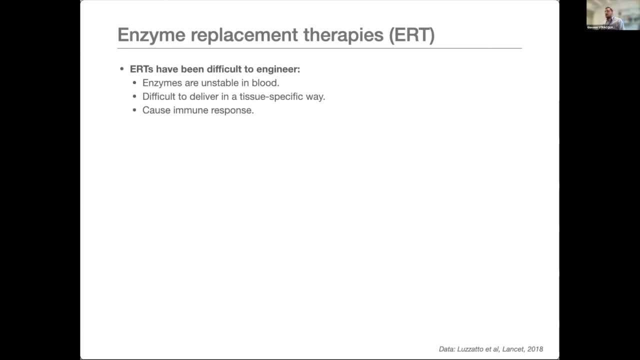 difficult to engineer. The enzymes are unstable in blood, They are difficult to deliver to tissue specific way and also causing new response, which is very important. But also they are difficult to manufacture because usually you use mammalian cell lines which are typically prone to. 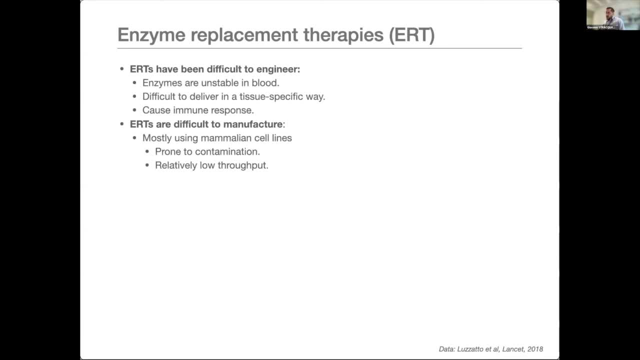 contamination, but also they have very low throughput. So, of course, all this taken together is posing a really big challenge to the healthcare systems across the world. The solution for now is that these drugs are basically categorized as orphan drugs, which are: 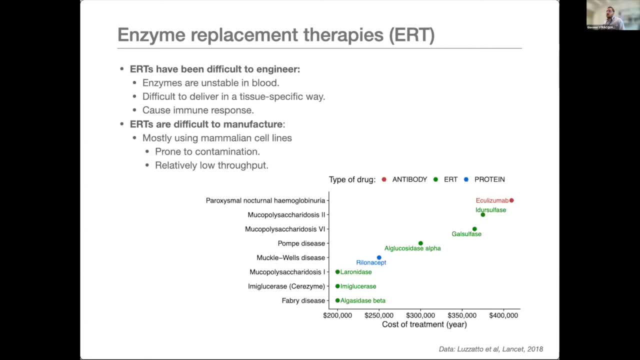 of course, some serious side effects, meaning that their cost has skyrocketed in the last 20 years or so. And if you look actually at the orphan drugs, the top, the most expensive one, that's six out of eight that actually are ERTs. So we got to sort of fix that, if you want. 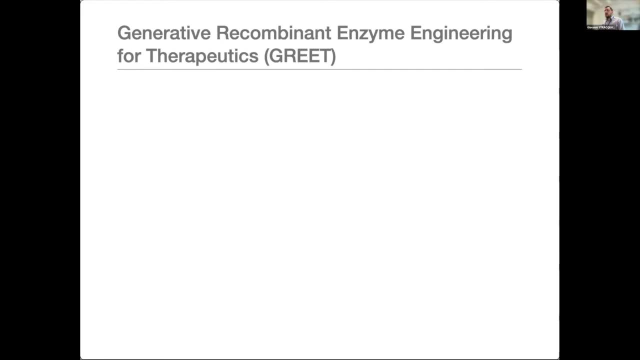 And I just started in January, the RIP project, which aims at doing three things in this area. First one is developing generative methods to design better ERTs. We want to also establish a sustainable platform for ERT manufacturing And we also want to release everything as an open source. 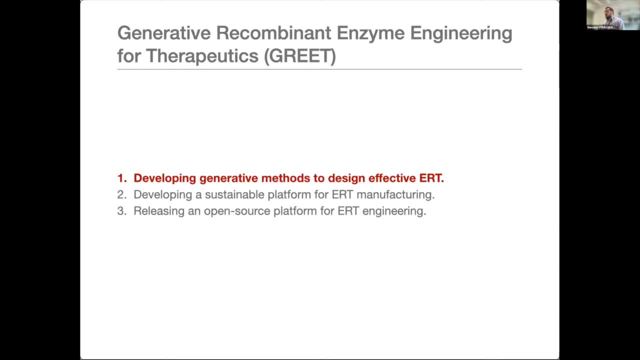 platform because we think this will enable treatment for other disease in this area, And I have to thank the UKRI EBSRC for giving the opportunity, through a fellowship, to work on this for the next four years, but also my industrial partners who have been very supportive. 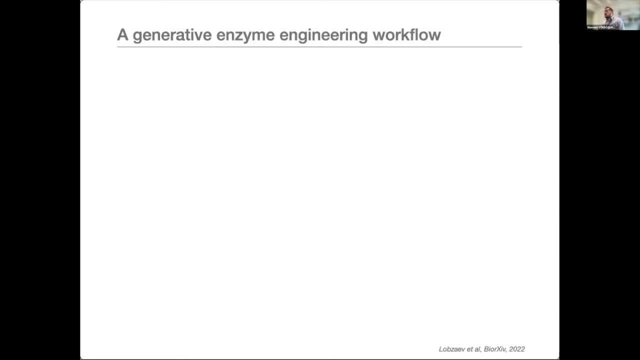 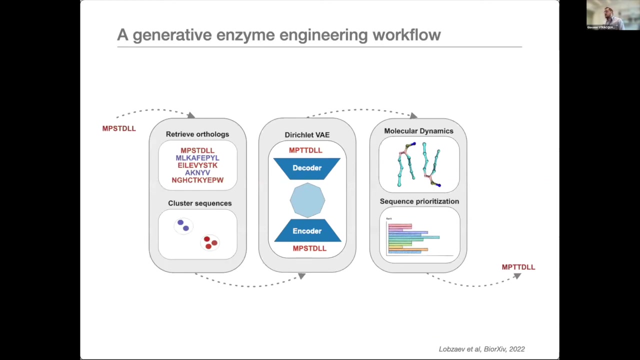 So how we actually engineered these enzymes, I'm not going to cover the details, unfortunately, but Procreate is coming out, has been submitted to BioRxiv, so it should be out today or tomorrow, And the idea is that you take a wild type sequence: you retrieve orthologs, 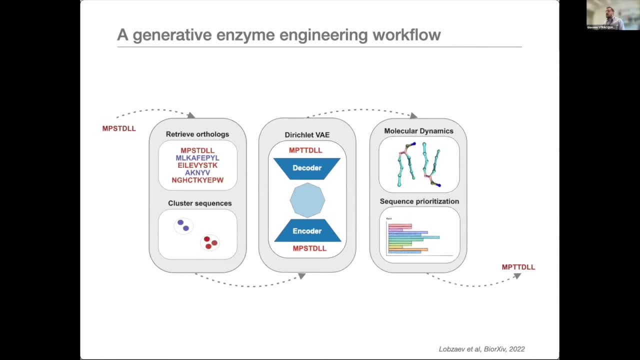 you cluster the sequence to build data sets that we can use to train our machine learning model, which I'll talk in a bit, And after that we use it to design new sequences which go through the sequence, which go through the sequence, and then we use it to design a new sequence. 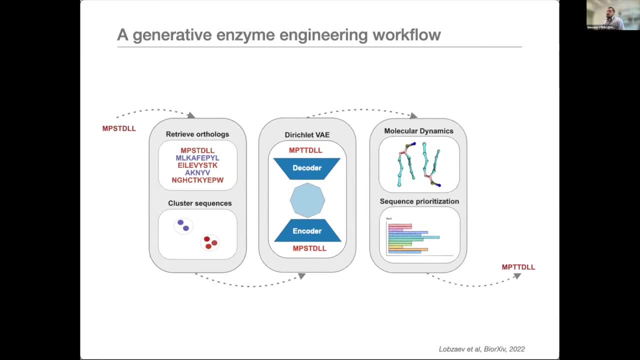 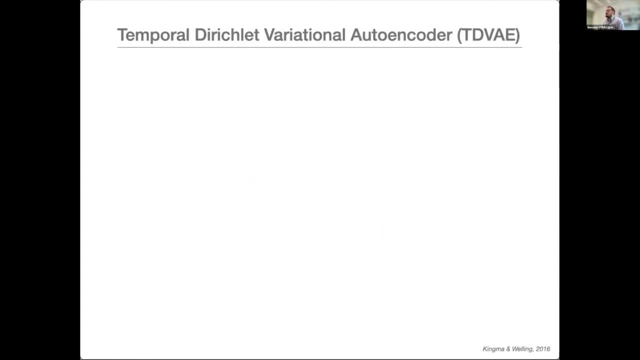 And so when we talk about machine learning driven design of proteins, we are really talking, in our case, about variational health encoders. So what we think is that enzyme engineering really means learning how to sample the protein design space to identify the amino acid sequences associated. 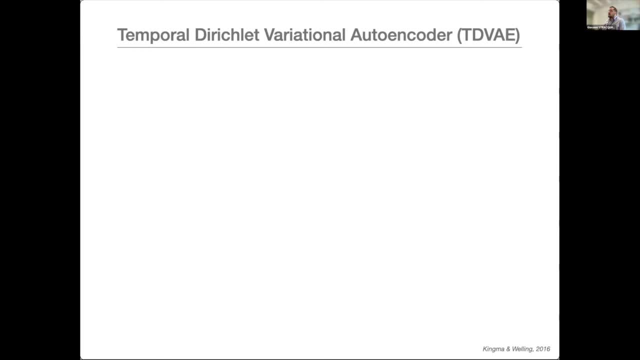 with the desired catalytic function, And our hypothesis here is that this design space is a statistical structure whose functional form, of course, and corresponding parameters are unknown, but we can learn them from the known sequences in nature, And so what we think is that we assume 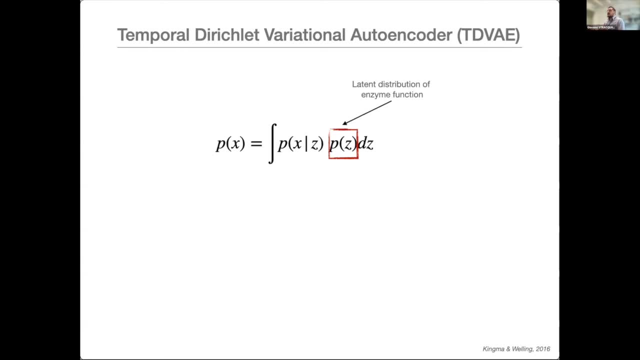 that the probability of observing a given sequence depends on a Latin distribution, so of unobserved features that Basically condition the probability of observing any sequence in this space. So when we look at this, we can replace this Latin distribution with one of the parametric that we routinely use. 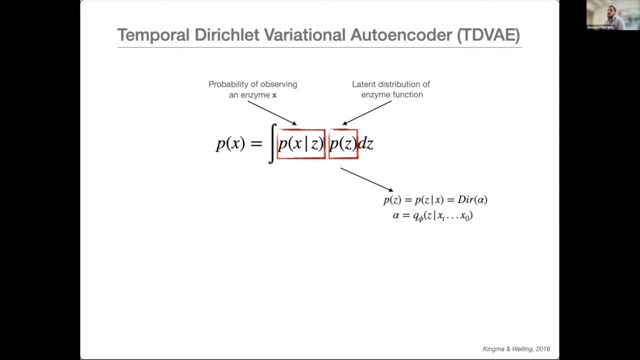 And I'll talk about the one that we are going to use here- And we are going to model the proteins that we can generate depending on these values, using the language models. So typically these models are very difficult to fit, if not impossible. 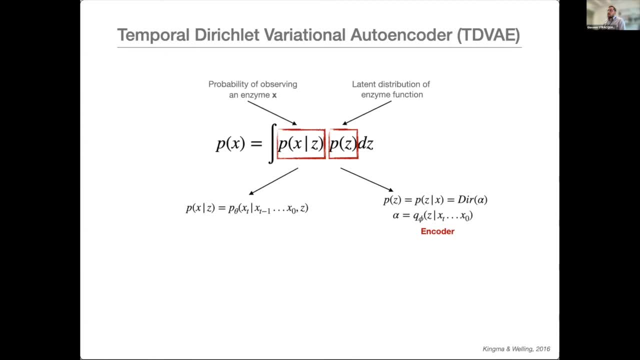 So. So we try to get around that in different ways, And we use a recognition model that we call the encoder, so that we know which distribution parameters associated to what we know, the observed sequence, And then we use this other model to decode this numerical value. 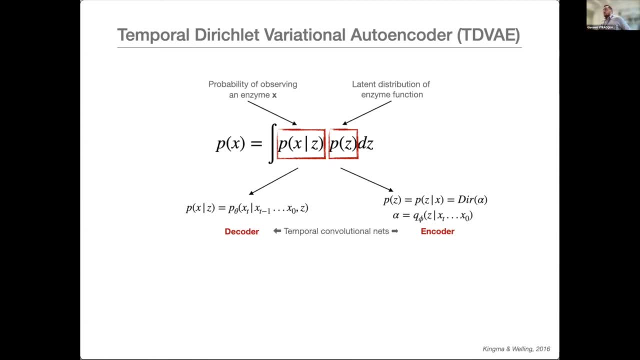 into a natural sequence. How we do that: We use temporal convolutional networks which allow us to deal efficiently with the biological sequences and text in general. And How you fit this model, which sounds really complicated and it is. We use stochastic variational inference. 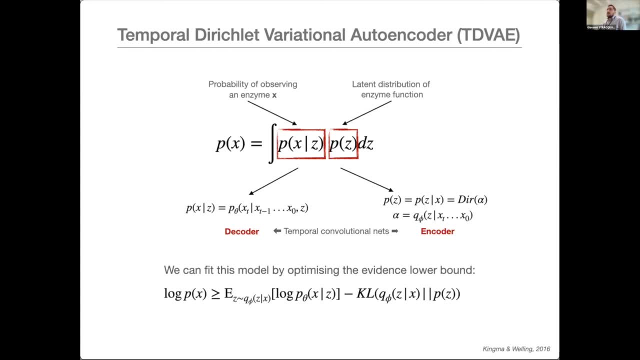 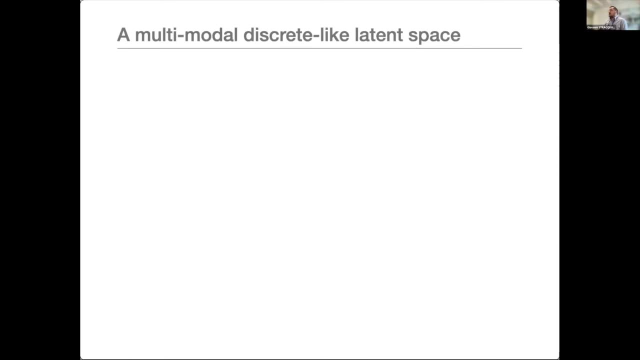 And specifically, we optimize the evidence logger bar. So when it comes to modeling the Latin space, so the features inherent to the proteins, we argue that this is a very important factor when it comes to generating functional proteins. And in the literature, the common solution. 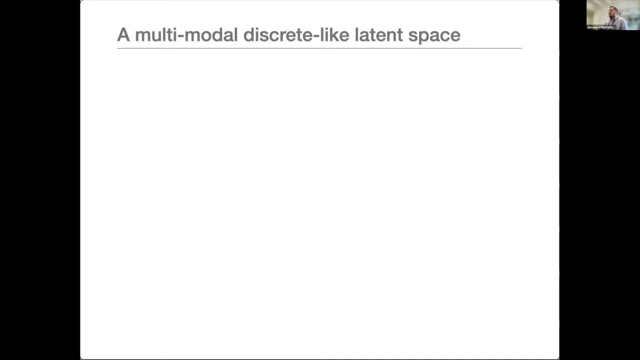 is that people use a Gaussian distribution, which is not really well suitable for this task, because it's difficult to model the multimodalities of the protein design landscape, And if you look here, for example, this is a very well-known picture. 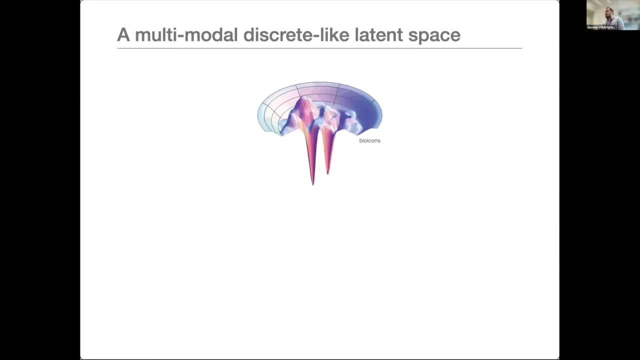 We thought which distribution could be better suited for modeling this scenario And we turned to the Dirichlet function which basically what it does is modeling multimodalities as a function of an alpha parameters And And with this, by modulating these parameters. 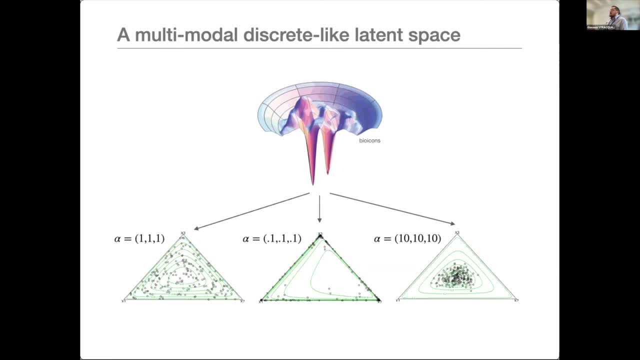 we can actually model different Bayesian over-attractions and different protein conformation in a very principled way. So this is one of the introduction that we did in the variational out-encoder framework, And we think this is kind of the secret sauce for our results. 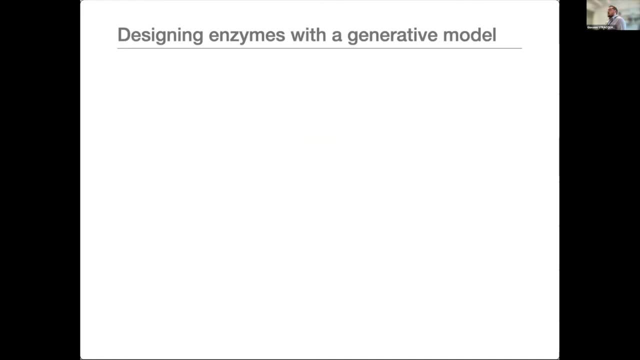 But what I think is more interesting from an end user perspective, how you're going to design the actual sequence, how you're going to get that. So we have two strategies. One is called prior sampling, which basically generates a random number from a prior distribution. 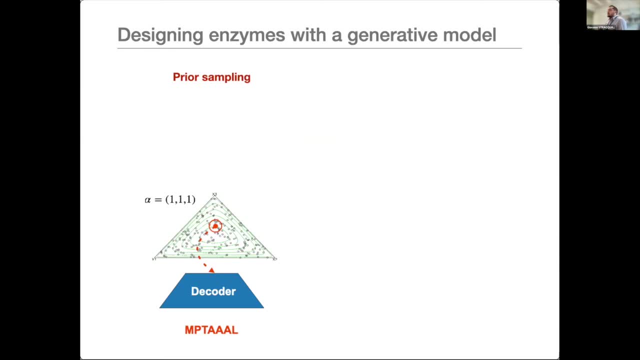 for the Dirichlet And we run through the decoder And this fits out a sequence that will look like one of the protein that you have seen in the training set. So this is important. It's more like the novel design, if you want. 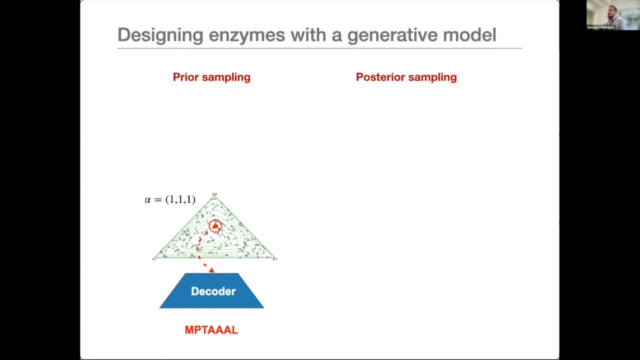 But if you want to generate variance, what you're looking at is what we call posterior sampling, where we start with a wild type sequence. We run through The encoder, We get the region of the design space that comprises this protein And then we sequence in this neighborhood a new value. 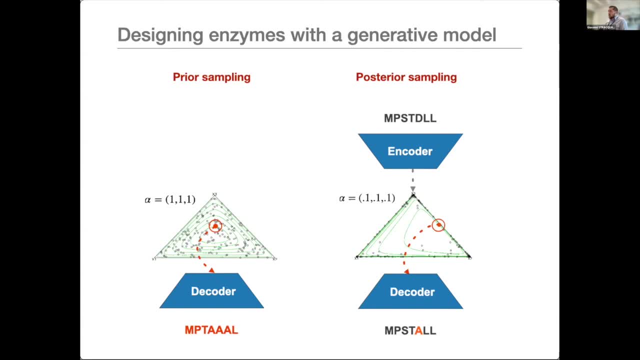 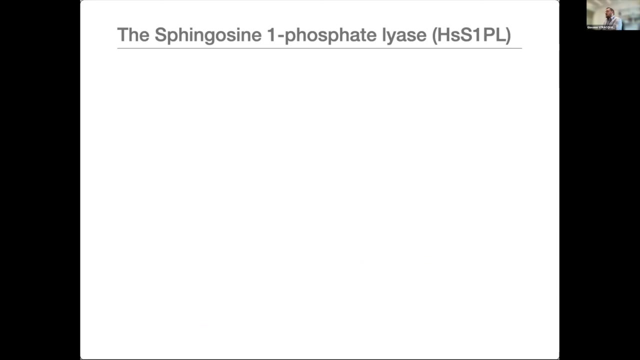 that we can decode And, basically, what we hope to find is a sequence that is very much similar to the wild type, but with a few mutations in it. So we use this approach to start working on sphingolipids, which is one of the class of lipids that we like. 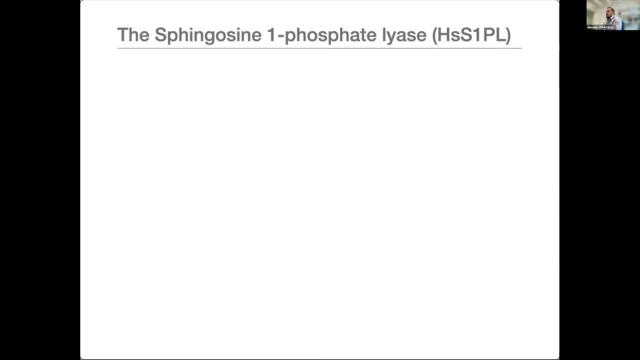 The most. they are very important for especially structural roles in the cellular membrane. There is one that is particularly important. It is the sphingosine 1-phosphate, a key molecule whose metabolism is closely regulated, And one of the enzymes that is particularly important. 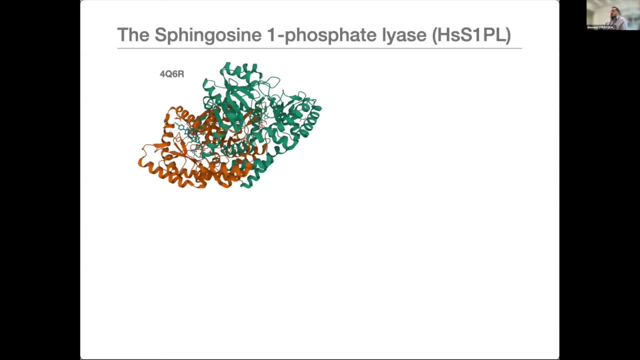 is that the great S1P is the paradoxal 5-prime phosphate dependent S1P which we are really interested in And, as you can see, this is a tight pocket where the PLP binds. The problem becomes when you get a mutation in the gene encoding. 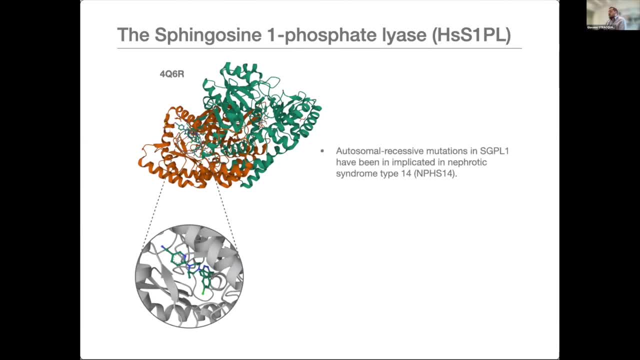 for S1PL, which has been only recently shown to associate with the nephrotic syndrome type 14.. And the current solution that has been explored is to develop an enzyme as a replacement therapy that can overcome the kidney failures with S1P. 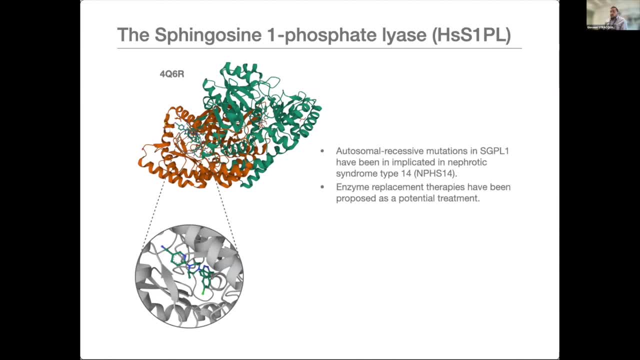 Thank you, Thank you, Thank you, Michael, Thank you very much. Thank you Very good. Thanks a lot, Michael. That's a very good point, And we also have some information from the last slide that you gave us about a variant that has been used with S1P. 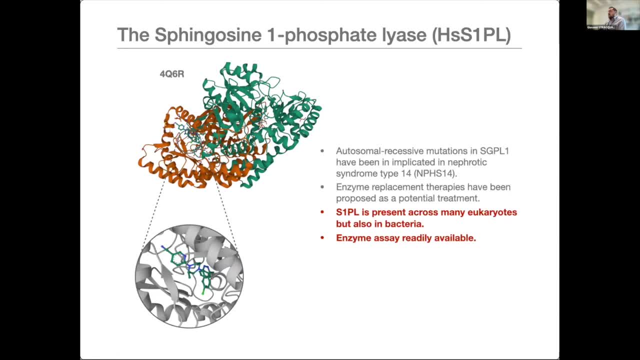 in our lab for most of the cases. So this is a different case that we are starting to think about And I will just show you a few case that we have used with S1P in our lab, And the first case is a variant that 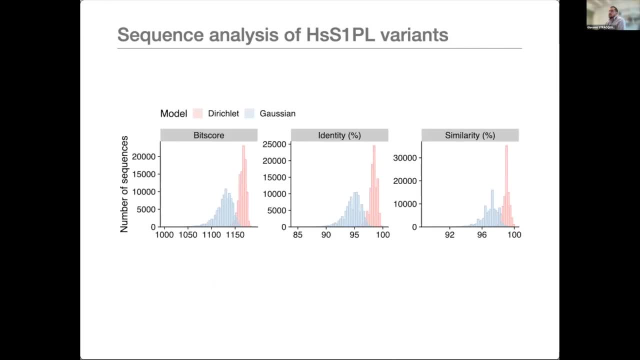 is present in our lab in the course of what is described now as a contraindication of legendary S1P in the TCA, And what you see in your slide here is the bovine retinopathy, Francesco D' As one pl violence, as you can see from this plot with different type of metrics, but also when you look at this new sequence, is you want to make sure that they still retain the functional properties of the wild type, just to 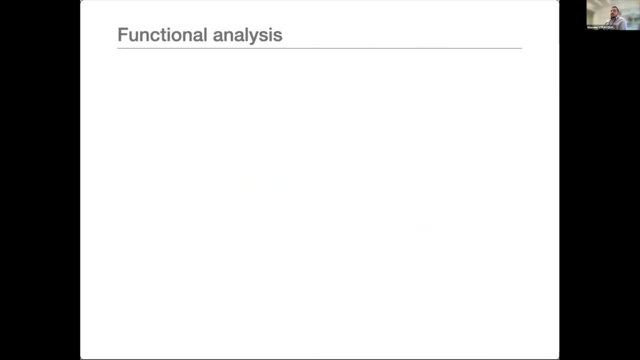 Francesco D' Somehow have a proxy to say that they are functional, Francesco D'. So how we do that? we first of all look to whether our new sequences retain the catalytic residues, which is a nice in that position 353 and all of them, as you can see on the right plot over here. 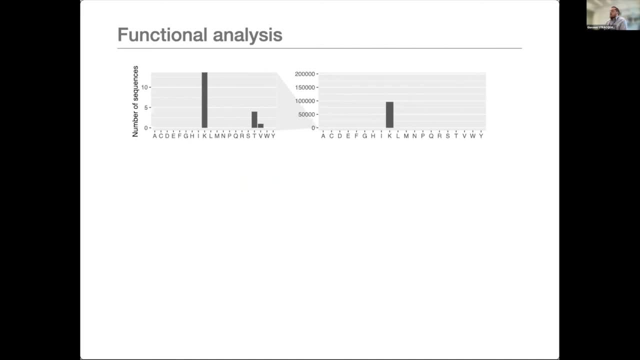 Francesco D' retain the lights in, except for five sequences, which changes to training and Bali. when you actually look at different Francesco D' indicators of protein properties, you will see that pretty much whatever we generate from the posterior distribution with our strategy actually retain the same or gravy instability index and is electric points. 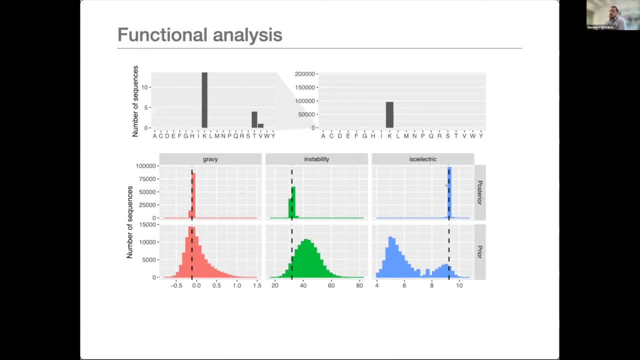 Francesco D' That we see for the wild type of which is represented here with the dash of light. so everything seems to be Francesco D' pointed to the right directions at least, and the nice thing to note here is that if you look at the samples, that is, that we generated from the prior, we see pretty much a big variations in this properties. most of them are unfoldable, probably, or 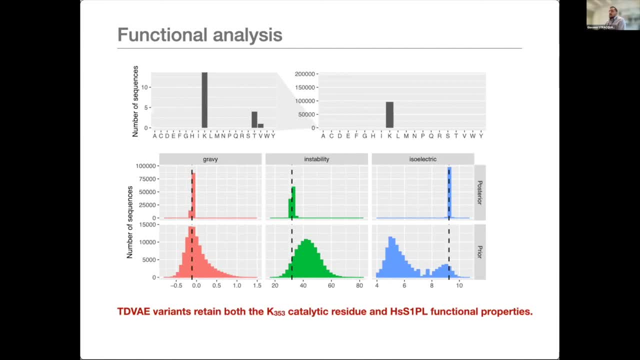 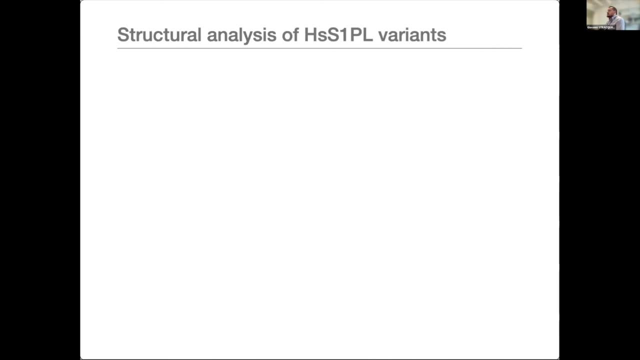 Francesco D', Something that you cannot have been the solution. so that's really showing that somehow our method is working, Francesco D'. Of course, at this stage it's all about sequences, but we know that structure is really important. so Francesco D' Michael did an excellent. 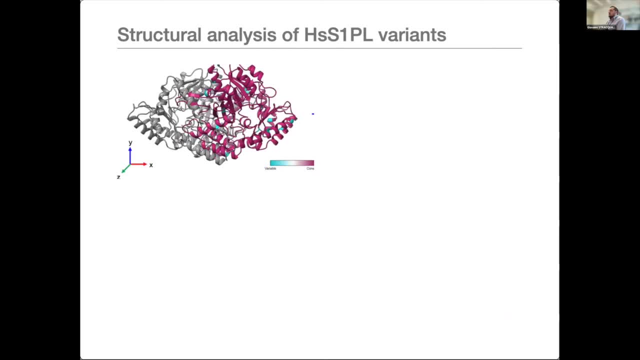 Francesco D' analysis at the structural level, where we mapped out all the limitations, is reduced by our machine learning methods on the nativity structure of s1 pl- human Francesco D' And we find basically that everything is in or around. the quality of the regions and the pocket where a plp binds is actually very much concerned, so this is really reassuring that. 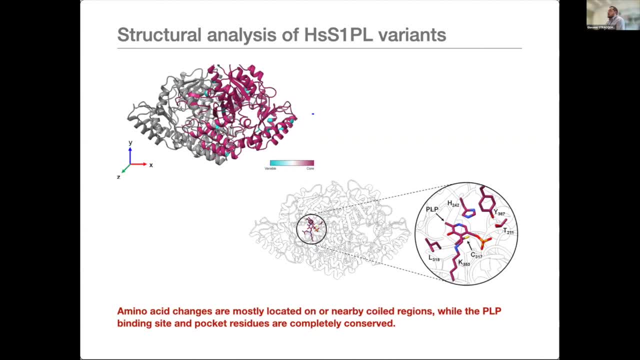 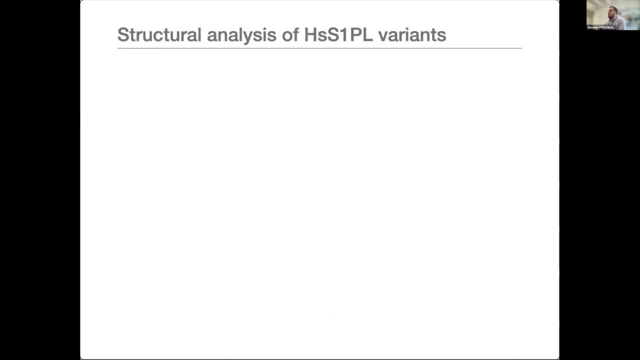 Francesco D'. Pretty much, our method is somehow learning to not touch the functional region of this product. so of course we wanted to Francesco D' Go further and Francesco D' Study how stable is the broadening over time? we did molecular dynamics, see the simulations and what we tried to see he's our, our proteins above as a function of the rms, the at each time step of our simulations. if you look at the wild type here. 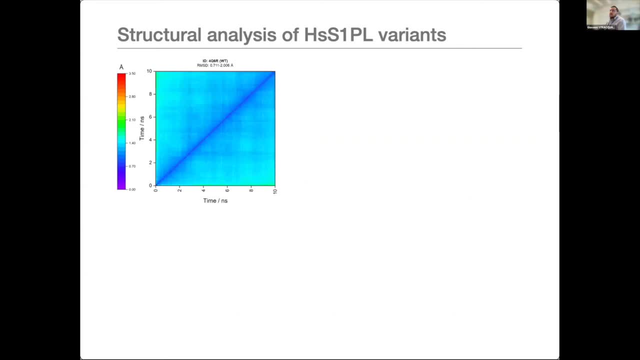 Francesco D' This is the so called the to the rms, the plots, you will see that the problem is very stable. but if you look at the Francesco D' Our variants, that we selected the pretty much a random, we did not be in between. 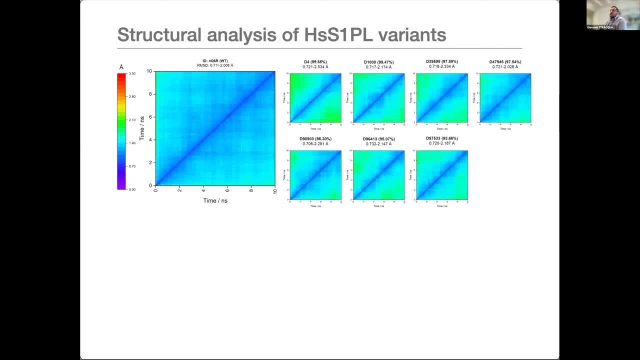 Francesco D' 90% and 100% similarity with the wild type. we see quite a wide range of of our changes in the stability of the structures, and there's a one important thing to note: that if we pick the Francesco D' variant, which is the most similar to the wild type, is actually one of the most unstable, meaning that some of the mutations that we introduced actually where, even if they were just a few, were extremely dangerous, whereas something that is a little bit more divergent. 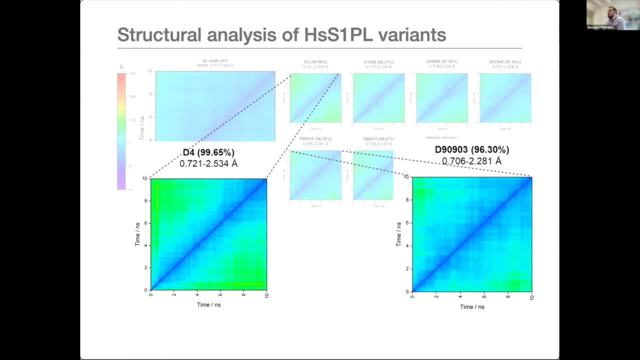 Francesco D'. Like here, Francesco D' it's actually more stable and it's probably one of the candidates we are bringing into the lab. so, long story short, what it tells you is that you cannot, just, Francesco D', Use a sequences to drive your design. about actually using up filtering. step based on structure will help you drive your designer towards more functional regions of the design space. 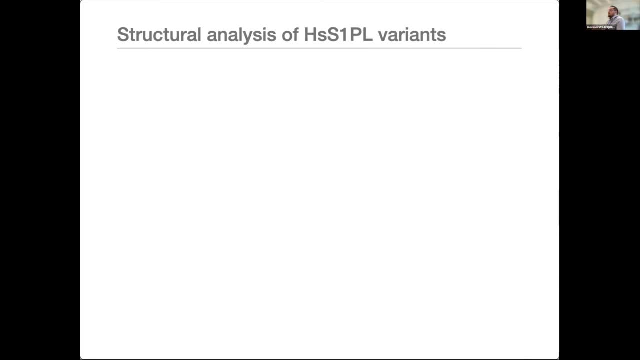 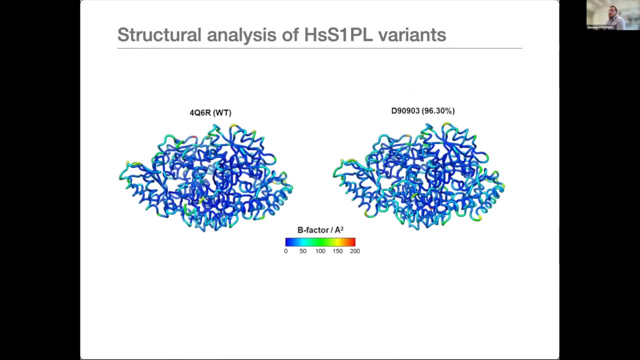 Francesco D'. And finally, since we have seen the most of the structure is somehow more flexible, Francesco D', The wild type. we did some factor analysis. this is the wild type and when we compared with the, what we think is the top candidate, we see that actually the most flexible regions are in the periphery of the of our molecule, which is kind of what we want. 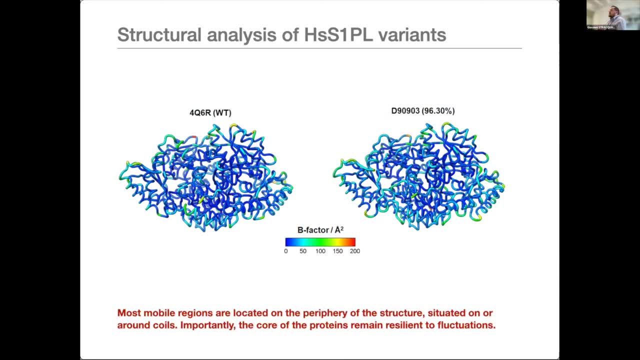 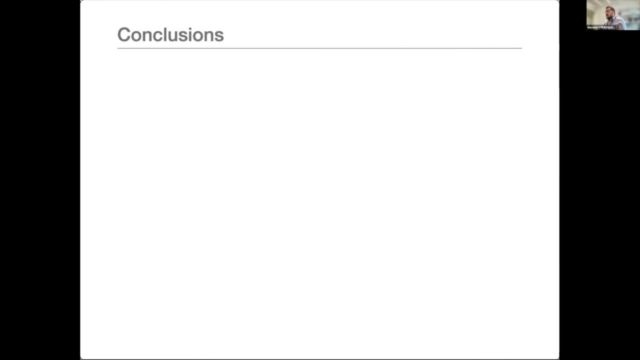 Francesco D', As at least we know that the structural component of our plp binds is tightly packed and it's very much structurally concerned. so this is where we are and we are moving into the lab to test all this, Francesco D': New enzymes in e coli or potentially is the, depending on which one reacts, better, I would say. and what we quickly realized is that 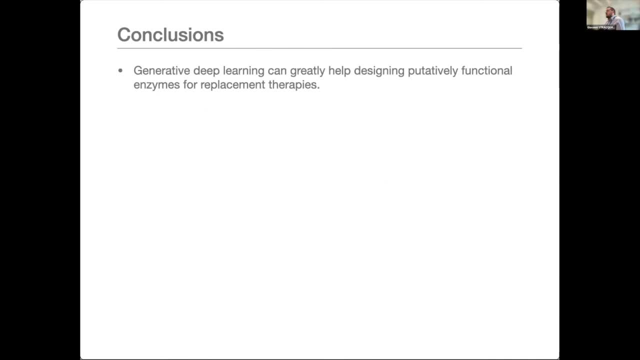 Francesco D'. generative deep learning can really be a game changing tool for designing the artists Francesco D' And what we think is going to happen is that we will be the position of developing targeted libraries. that will speed up tremendously the time to bed on this therapies. 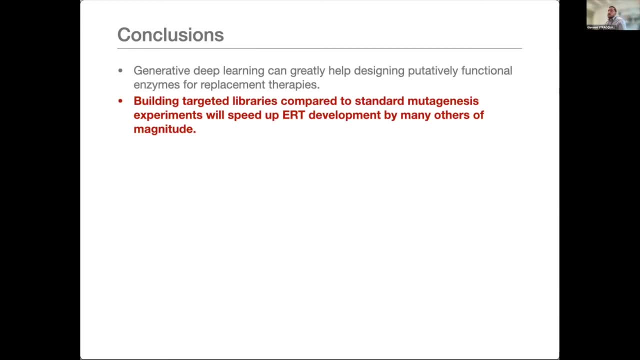 Francesco D' Compared to stand Francesco D' The random mutagenesis experiments. of course, it's not all gold what we see, but there are still mathematical and experimental challenges that we need to address, like, for example, learning from only few.